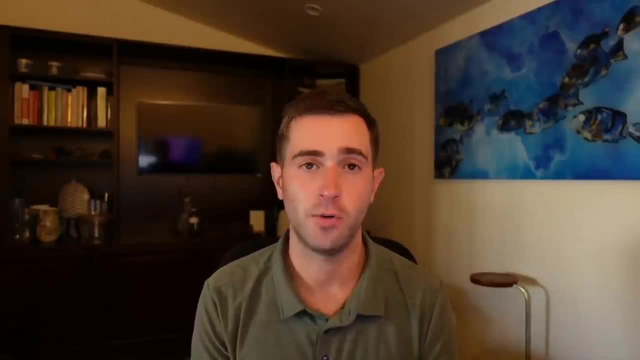 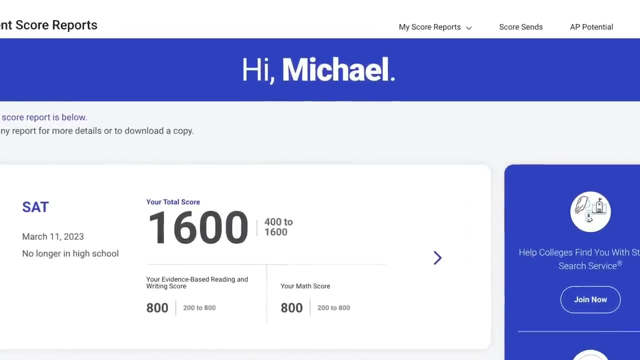 Hey, Mike from PrepPros here, and for those of you who don't already know me, I'm on my ninth year of working full-time in test prep. I've scored perfectly on the SAT myself. I've helped students score perfectly and many score in the 99th percentile, and I just published my second SAT. 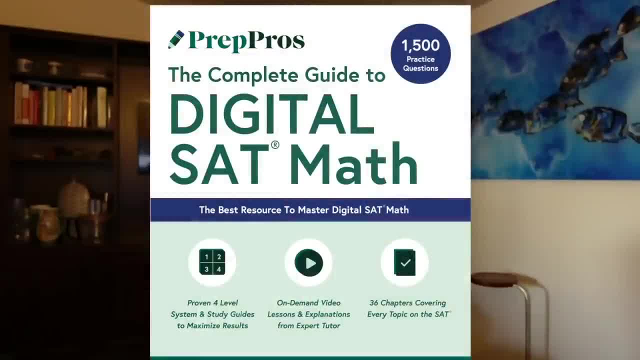 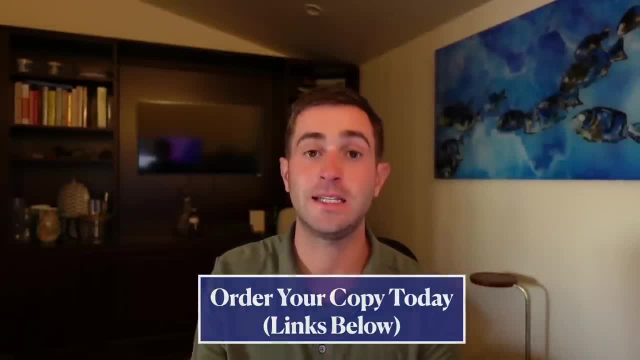 math book completely updated and revamped for the new digital SAT, which I think blows anything else out of the water. So I know a thing or two about helping students do really well on the SAT. so in this video we're going to run through a super helpful exercise for you to ramp up. 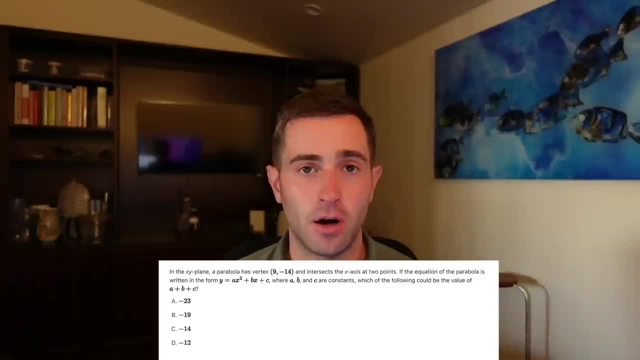 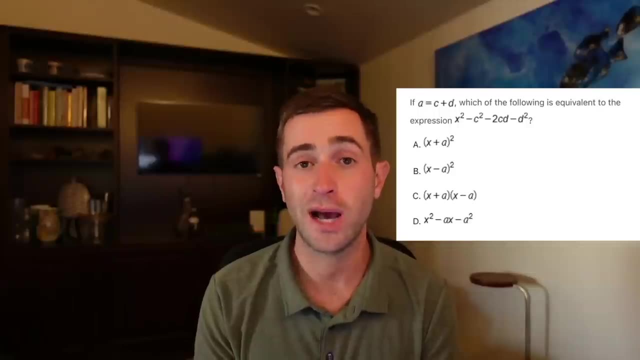 your digital SAT math skills. We're going to take a look at the 10 hardest questions that College Board has released for the new digital SAT and I'm going to teach you some really helpful content, tips, tricks and strategies, along with Desmos, hacks for how to take some of those very 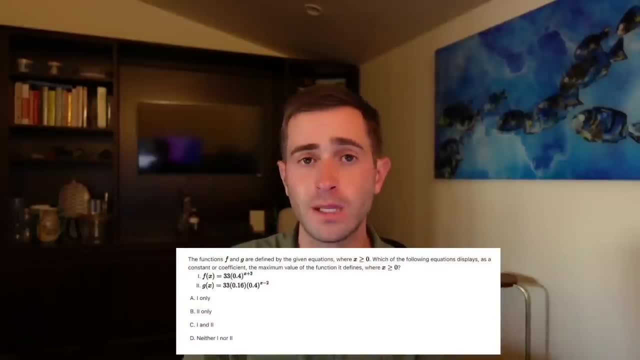 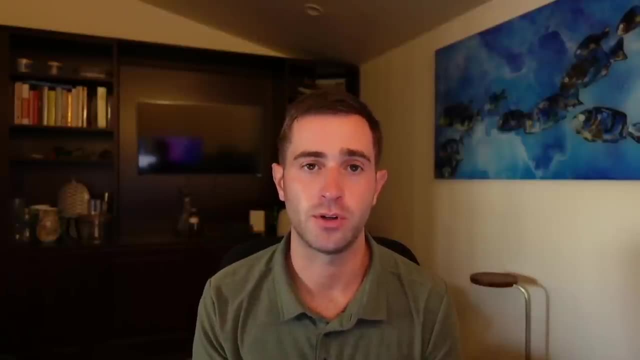 complex questions and make them far more approachable. At the end of the video I'm going to talk about some additional resources which can help you better prep for the digital SAT and get that perfect score that you're looking for. Function f is defined by f of x equals. 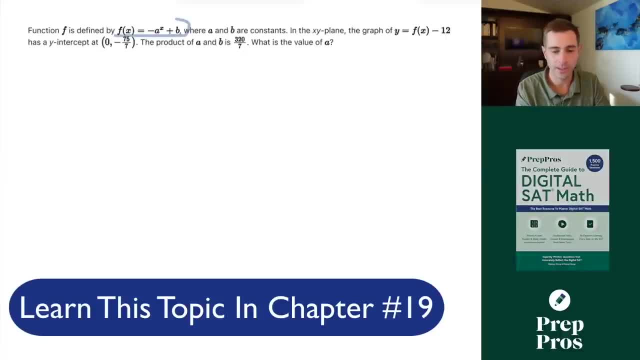 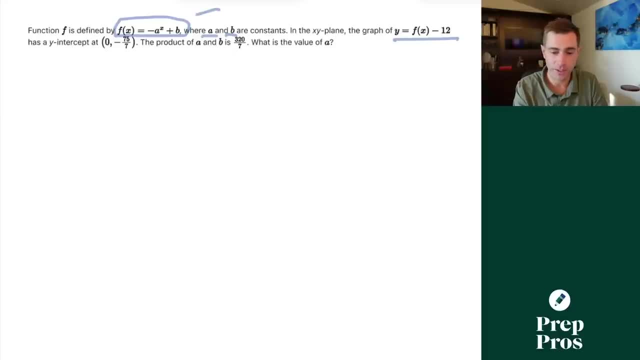 negative 8 to the x plus 1.. So this is going to be an exponential function where a and b are constants. in the xy plane, The graph of y equals f of x minus 12, so this function, shifted down 12 units, has a. 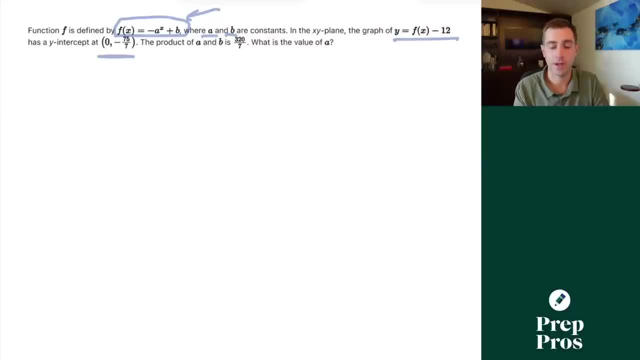 y, intercept at 0 comma negative 75 over 7.. The product of a and b is 320 over 7.. What is the value of a? This is a lot of information to try to wade through, but what we always want to pay attention to is if you get any of these really difficult, exponential questions. 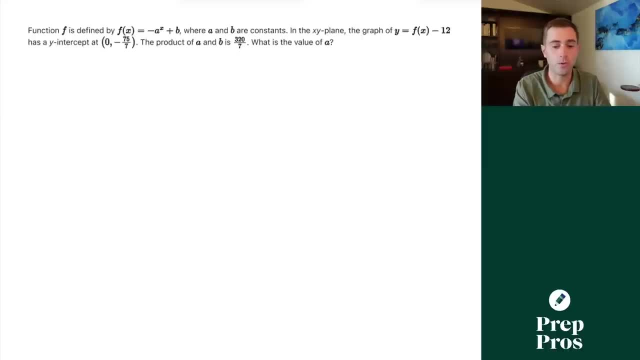 you're following the same series of steps we're about to go through. They're always going to give you a point that you can plug into, and what we always know is this first portion is our x value, the second portion is our y value. So we can just start to plug. 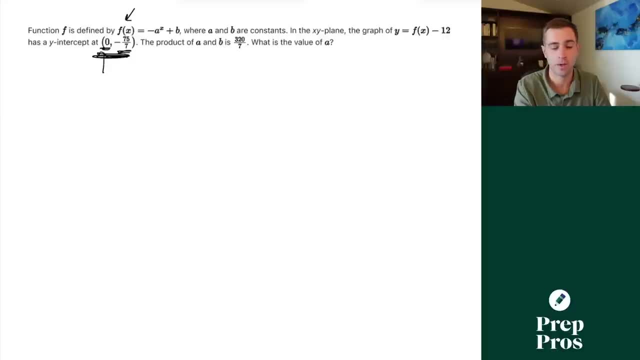 this in and we want to remember f of x is the same as y, So we can go ahead and rewrite this as negative. 75 over 7, plugging in for y is equal to negative a to the 0 plus b. 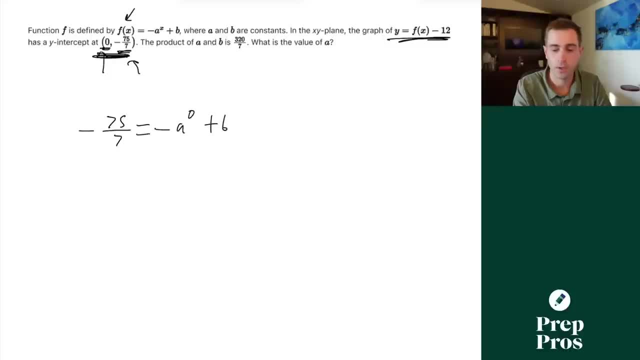 but since the shifted down function had this point, we also have to bring in our minus 12.. Now, from here, anything to do with f of x equals negative 75 over 7, plus b equals negative a to the 0 plus b. but since the shifted down function had this point, we also have to bring in our minus 12.. Now, from here, anything. 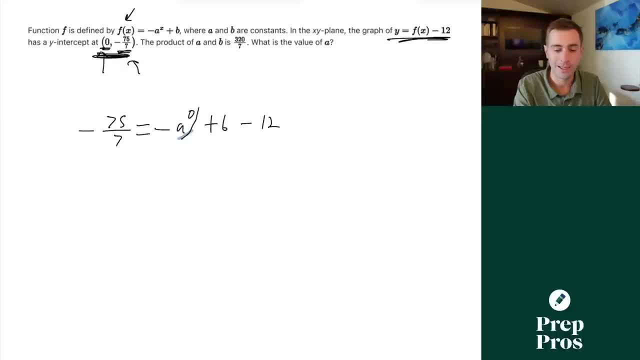 to do with f of x equals negative 75 over 7, plugging in for y is equal to negative 75 over b plus 12.. So this is going to give us negative 75 over 7, you're going to get negative 75 over 7 plus b minus 12.. This 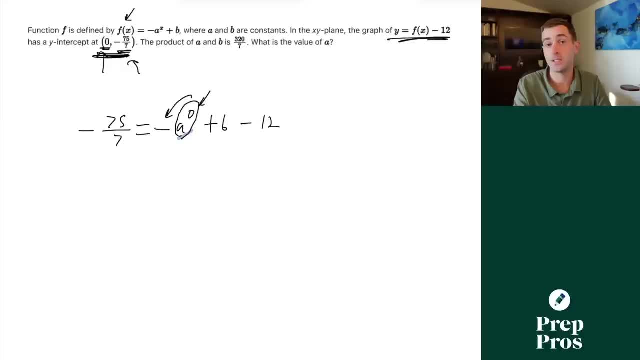 explain the. anything to the 0 is 1, but this is going to now be the same as negative 75 over 7 is equal to negative 1 plus b minus 12.. So this is going to give us negative 75 over. 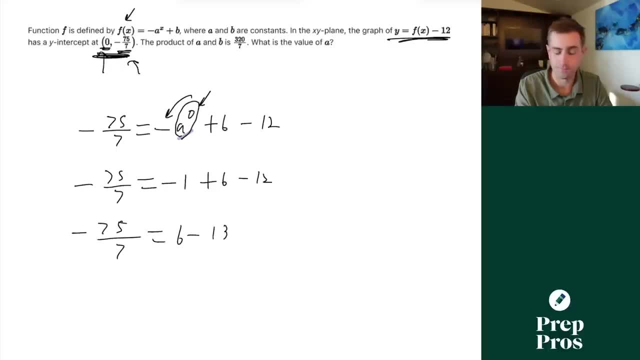 7 is equal to b minus 13,, which now means we need to add the 13 over 13 in terms of 7 is going to give us 91 sevenths minus 75 sevenths, it's going to be equal to b. so that's going to tell us that 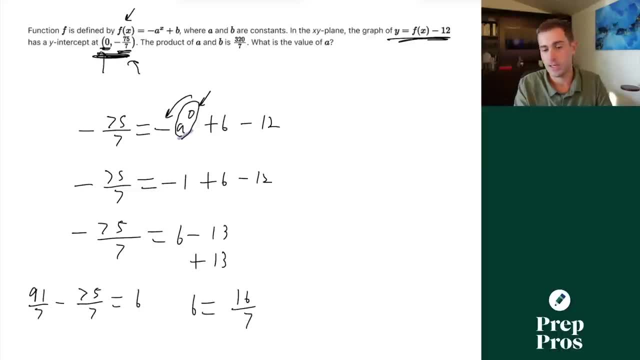 b is equal to 16 sevenths. now, from here we're mostly home free. the product of a and b is 320 over 7. well, now we just need to set this up is what we know is a times 16 over 7 is equal to: 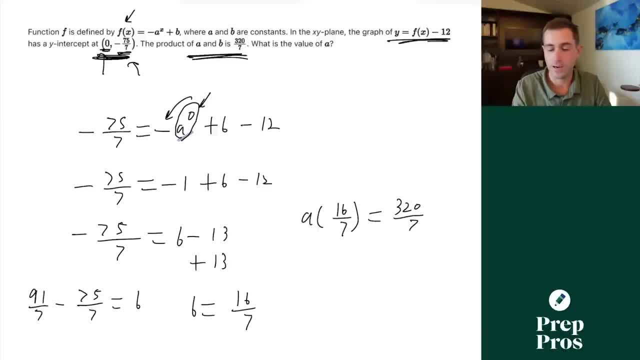 320 over 7. so now we can just divide both sides by 16 over 7. you can use your calculator here, or we can multiply by the reciprocal, which is the same as 7 over 16. our sevens are going to cancel out. 320 divided by 16 is going to give us our correct answer of. a is equal to 20. main point: 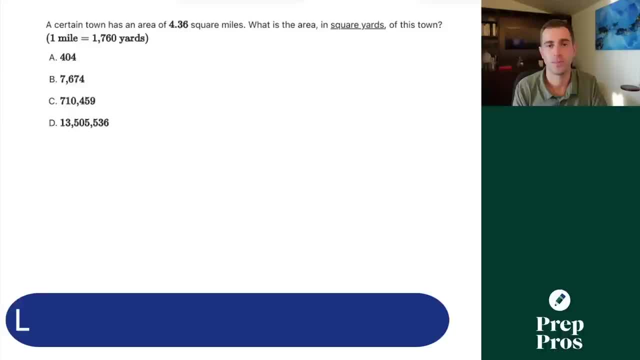 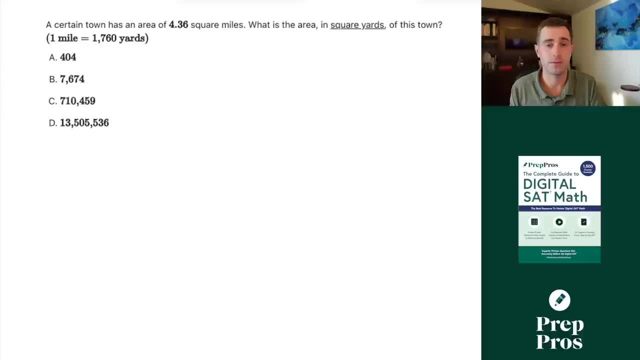 here. look to plug in the values if you get one of these on test day. now, not all digital sat math questions are necessarily correct. is time intensive- is the first one we went through- or is technically difficult to some of the really crazy ones we're going to go through later in the video. oftentimes they're hard because 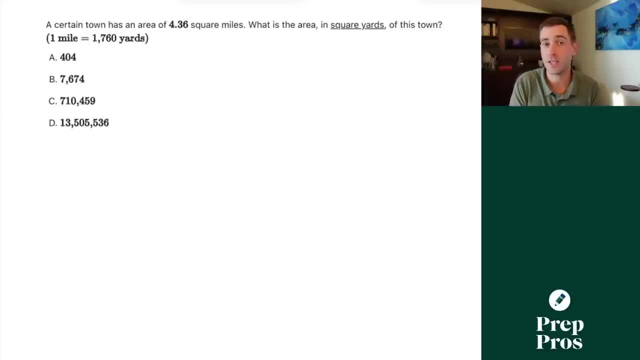 the sat knows you're going to make a common mistake and you feel like you found the right answer, and then you end up after the test realizing you missed it. so i strongly recommend to pause the video here. see if you can find the right answer. then we'll break this down together now, if you. 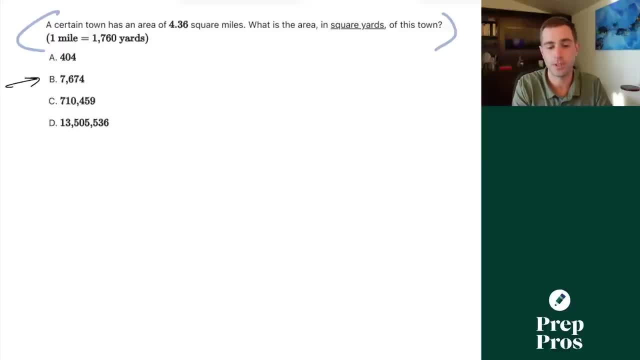 picked b, you fell for the sat's trap. so here we have a certain town has an area of 4.36 square miles. what is the area in square yards of this town? one mile equals 1760 yards, so this is a unit conversion question. the sat loves squared and cubed unit conversion questions because students 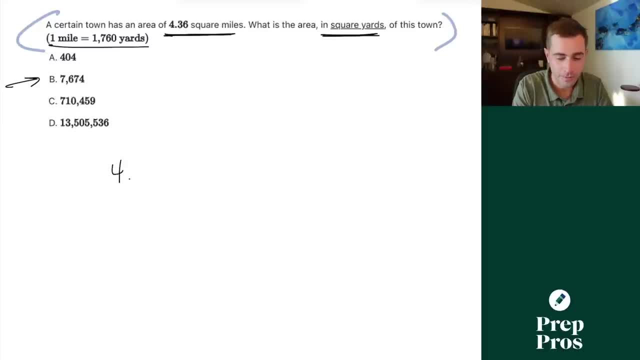 mess these up all the time. so what we can think about is: there's a few different ways we can go through this, but i'm going to do it one way that often feels simplest for students. so we have 4.36. this m here is just miles, and we're going to do miles squared, since it's squared miles. 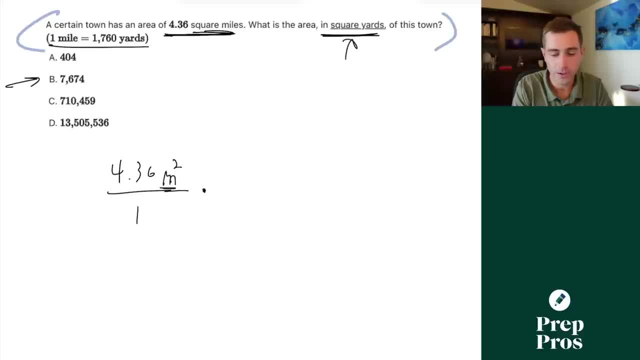 if we want to convert it to square yards. what we cannot do is just simply use our conversion factor and do 1760 yards over one mile. this is squared, so we need to square our conversion factor. so what we're really doing here is, instead of simply 4.36 times 1760, we're doing 4.36 times 1760 squared, and 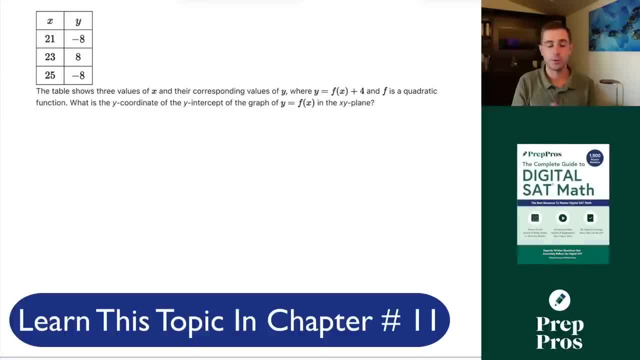 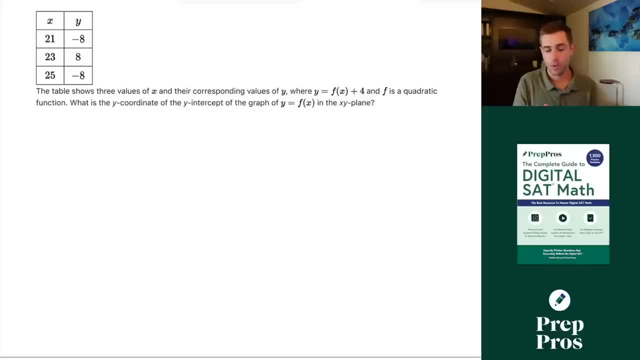 that will give us our correct answer of d. the table shows three values of x and their corresponding values of y, where y equals f of x plus four, and f is a quadratic function. what is the y coordinate of the y-intercept of the graph of y equals f of x in the xy plane? well, what this tells me is: i want to find the y-intercept of this. 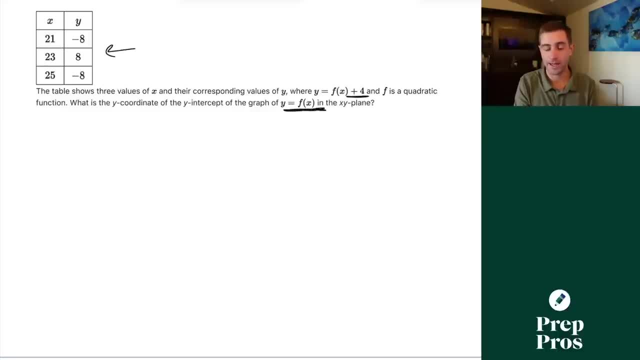 and then i need to subtract four from it and i can find the y-intercept of f of x, since this is shifted up four now. this is the first of the three quadratic questions we're going to look at. the sat loves quadratics for a lot of the really advanced questions. 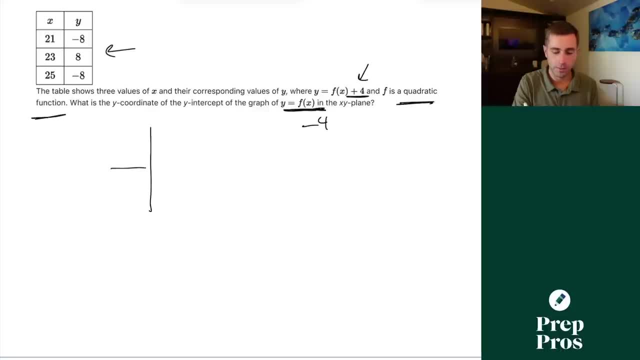 now there's one thing that's really important to understand so we can actually get started on this question, and this is that parabolas are perfectly symmetrical. so you might remember from math class, you have what's called an axis of symmetry, and if i drew this a little better, we'd have stuff. 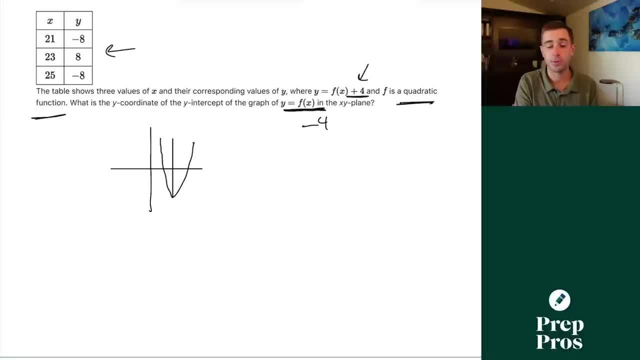 equally equidistant on both sides, but parabolas are perfectly symmetrical. so what this tells me is- this is my vertex, because as i go, two units to the left in two units to the right, i have the same values, and we're going to go over how to do this in desmos, so that visual will help you if this. 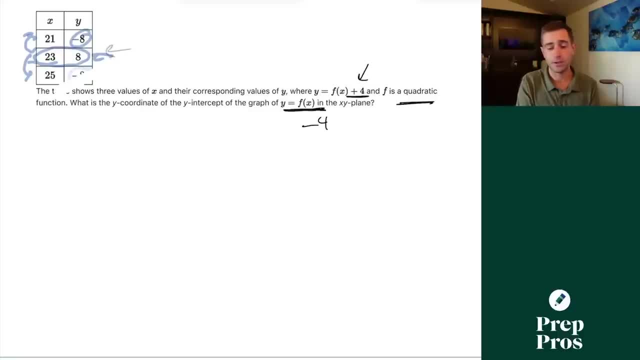 isn't clicking yet, but this gives us a way of understanding that our vertex is 23, 8.. so what this tells me is: i want to use vertex form to start this question, so i'm going to do: y equals a and our vertex form is: x minus h, squared plus k. we don't know our a value, but we know our h is. 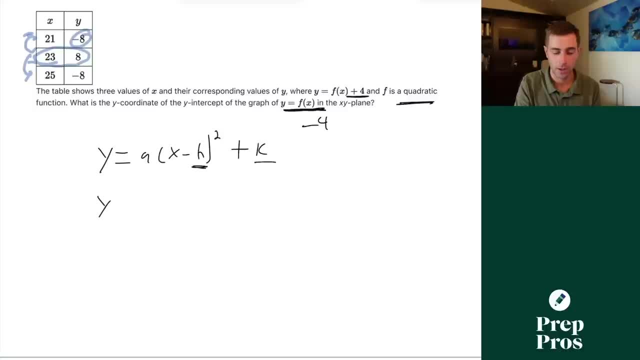 our x coordinate of the vertex, k is the y coordinate of the vertex. so we're going to do: y equals a times minus 23, squared plus 8.. now we're stuck because we need to solve for a. anytime we get these word problems, we're going to always have another point that we can plug in. we could plug in either of: 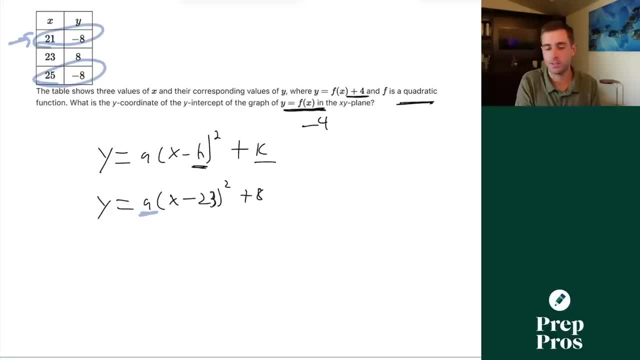 these points. i'm just going to go ahead and i'm going to use 21 here. doesn't matter which one we use, so i'm going to plug in negative 8 for y is equal to a times 21 minus 23, squared plus 8.. 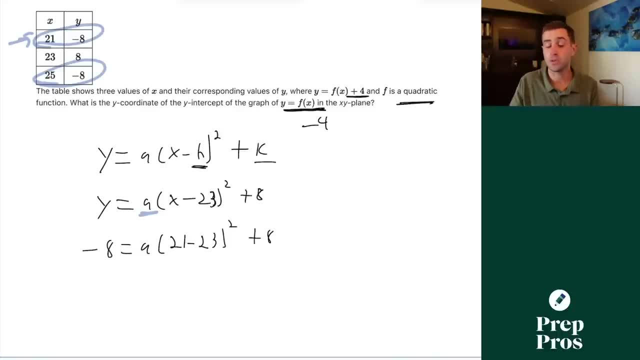 well, 21 minus 23 is negative 2. negative 2 squared is 4.. so this is going to give us negative 8 equals 4 a plus 8. subtract this over, we will get that negative 16 is equal to 4 a and this: 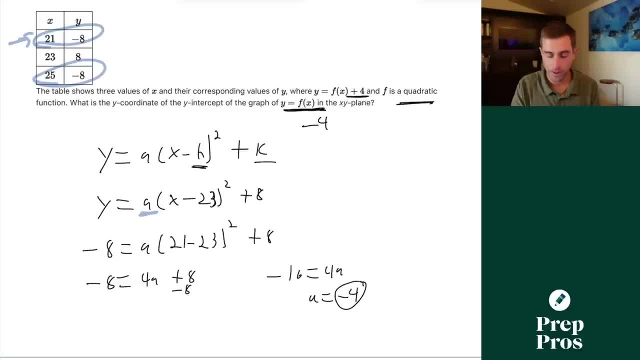 will give us that a is equal to negative 4.. now we know the entire equation of our parabola. so now we know that our entire equation is negative. 4 y equals negative 4 times x minus 23 squared plus 8.. now, if we're looking for the y coordinate of the y-intercept, 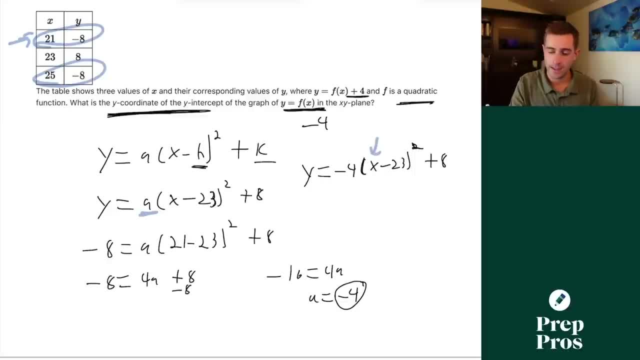 we always find our y-intercept when x is equal to 0.. so we just get to punch this in our calculator. we'll do: y equals negative 4 times 0 minus 23, squared plus 8.. so i'm just going to pop this: 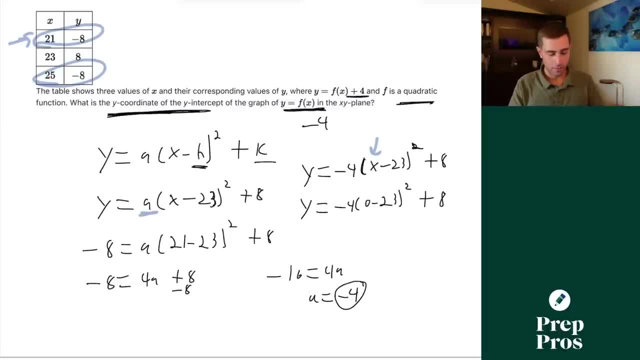 in my calculator now we'll get our negative 23. squared is going to give us 529 times our negative. 4 is going to give us negative 116 plus 8.. it's going to give us y equals negative 2108.. but this was. y equals f of x. 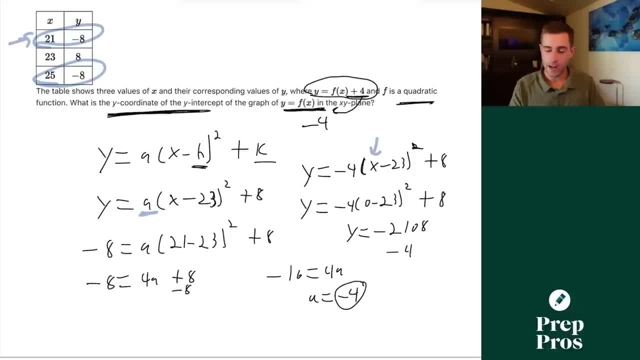 plus 4, and we're looking for f of x. so we need to subtract 4 from this and that will give us our correct answer of negative two thousand one hundred and twelve. but now we're going to jump on over into desmos and show how we could use that to actually solve this really hard equation. we've covered all the work in this video. if you haven't already, if you haven't really done so, be sure to subscribe to my channel and give this video a thumbs up. i'll ask you a question on how to solve the answer from here. so if you don't remember the first question, you didn't know what to do- then keep. 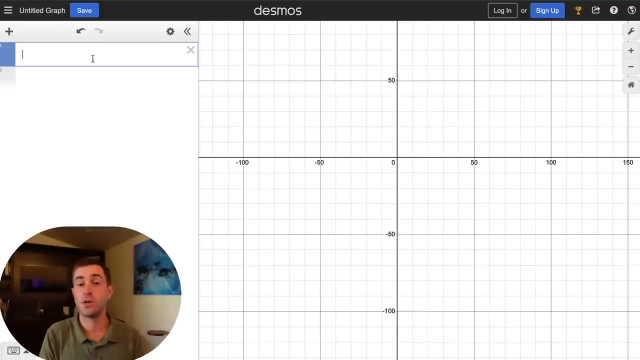 on reading it. now. there's three questions to go through. first question: we're going to asked to this really complex question, All right. so if we're going to use Desmos, we still need to understand the basic concepts of our vertex form and being able to spot using that principle of symmetry. 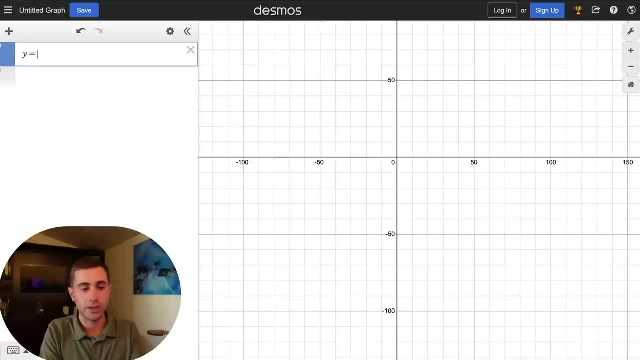 that 23 and 8 was our vertex, but we can. if we do that, we can write: y equals a times x minus 23 to the second plus 8, and we're going to click this add slider button. Now, what we also knew is we: 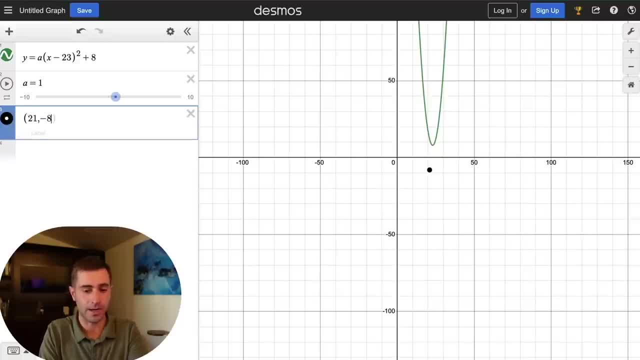 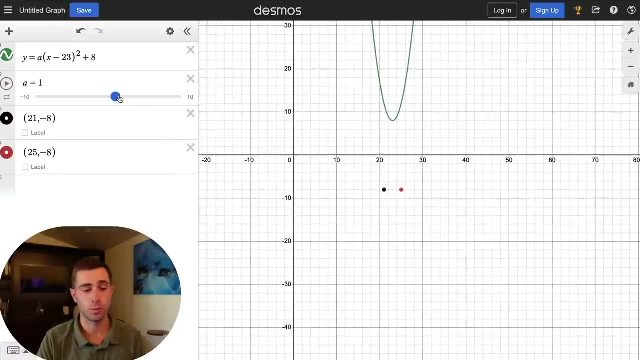 also had those two points of 21 comma negative 8, and we had that other point of 25 comma negative 8.. So here this is how we can actually use the slider to play a little bit of guess and check, because what we know is that parabola goes through those points. So now I can just play with the 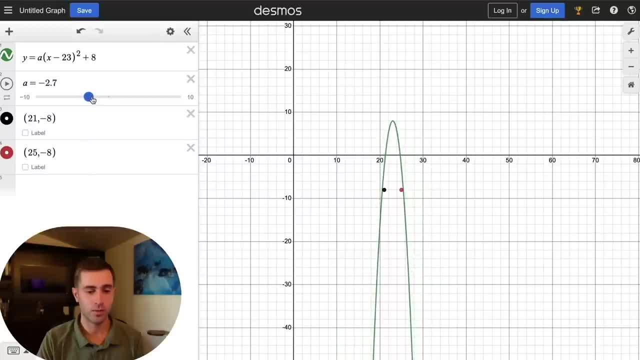 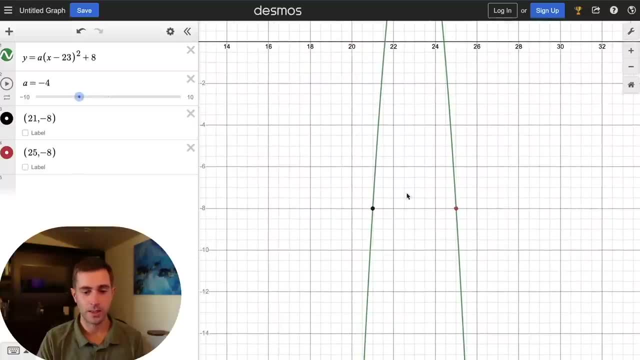 slider. it's going to have to be negative and I'm going to see where I go right through those two points here. So we're going to have to zoom in now. we're not quite hitting those points, but right there we have a point of 21 comma negative 8 and we have that other point of 25 comma negative 8.. 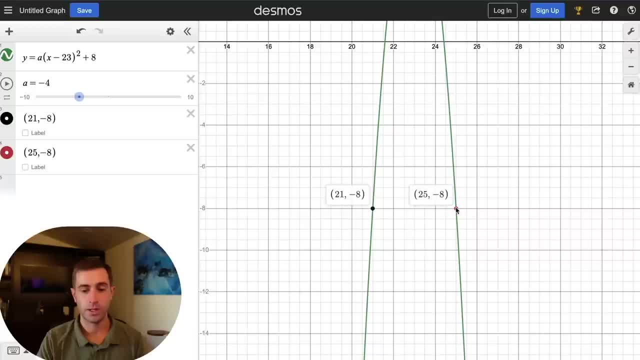 We can see we hit those points really nicely. so we'll get these kind of points of interest when we're actually intersecting. So now that tells me, okay, my a value is negative 4.. Well, now we need to solve for the y intercept, but we do also need to remember we need to subtract 4 at the end. So 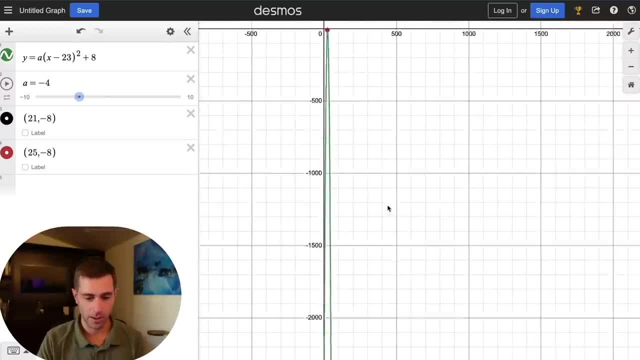 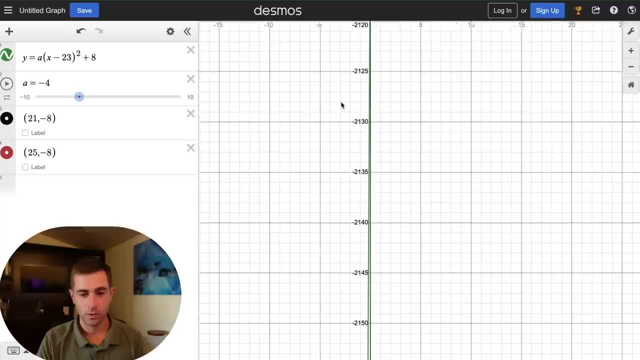 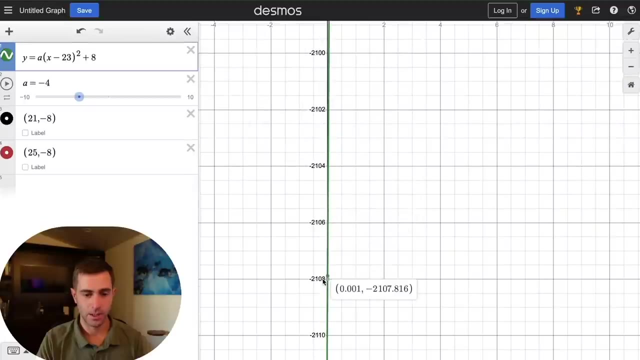 we're going to zoom way on out here and zoom out even further and we already know where we're intersecting. but if we didn't, we would just keep kind of coming down here and seeing where we get. this nice point of interest again, We should get one here where we get our 0. There we go. that was our 0 comma negative 2108.. 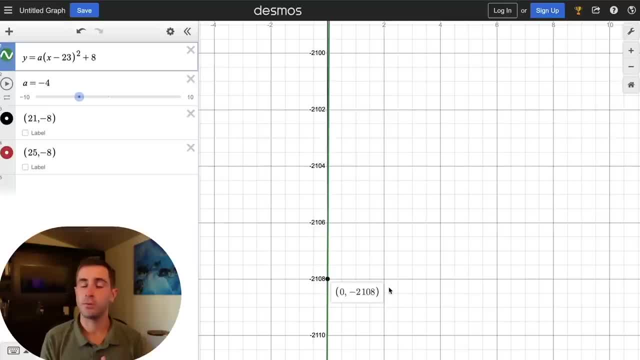 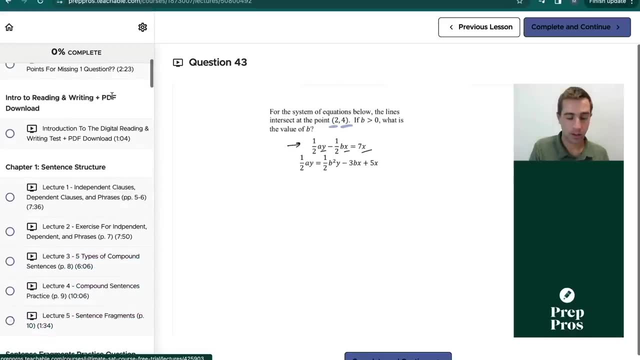 We would just have to remember to subtract our 4 at the end. We'd still be able to find that correct answer of negative 2112.. If you've been learning a lot in the video so far and you want to learn everything that you need to know to get a perfect 800 on the SAT math test, I recommend that you. 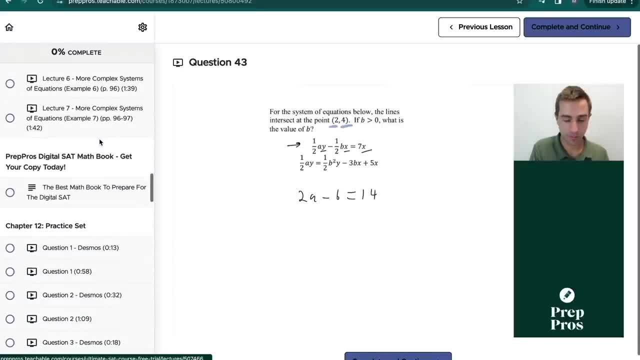 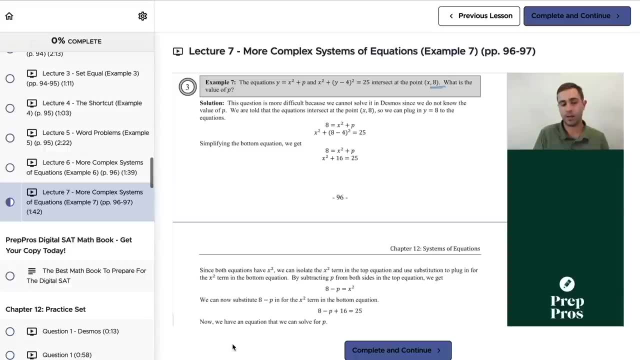 check out the free trial to my ultimate SAT course And there you're going to be able to check out the entire system of equations chapter from our brand new published digital SAT math book and you're also going to be able to access all of the lessons, explanations and Desmos hacks for the system of equations chapter. to teach you some of. 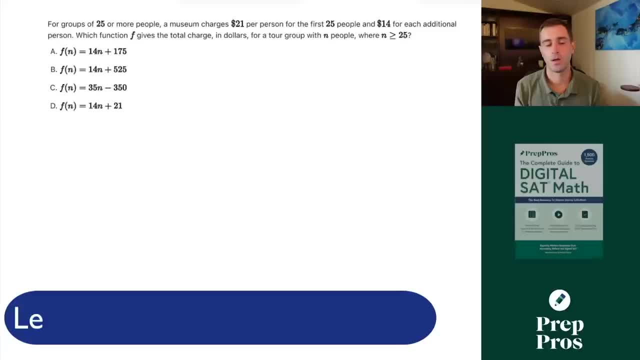 the most important skills to help you get that perfect. 800.. For groups of 25 or more people, a museum charges $21 per person for the first 25 people and $14 for each additional person, which function f gives the total charge in dollars. for a tour group with n people where n is greater than. 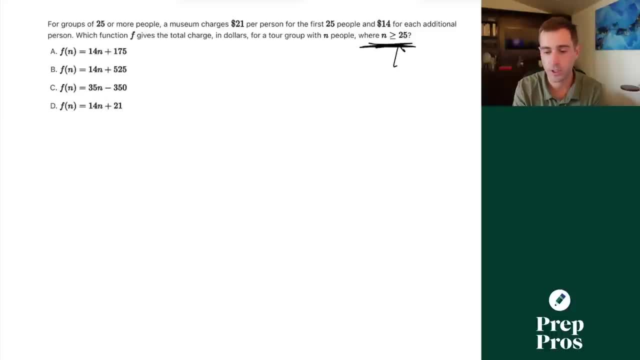 or equal to 25.. Now the trick here is that if you want to get a perfect 800 on the SAT math test, you can do that by using the Y intercept. So the tricky part is we're starting basically at 25 and we're 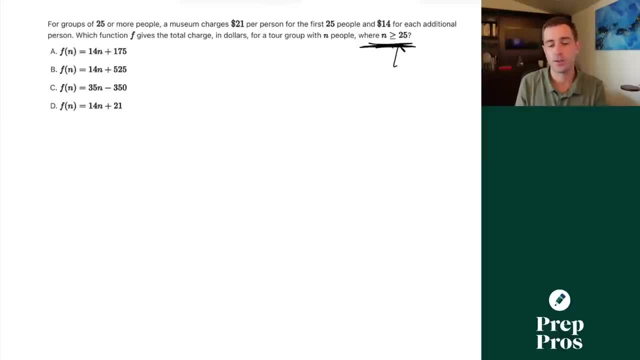 going beyond that, so it's almost like we've shifted the y intercept. There's a little trick for how we set these up, but once you learn it, they're quite easy questions to get right for being so difficult. First thing is we're going to multiply our whole first group, so this is our 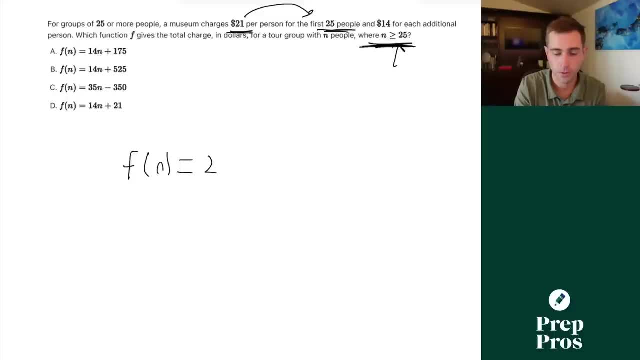 first 25 people at $21 per person. So we can do our 21 times our 25, plus the price of each additional person after that first group. so it's going to be 14.. Now here comes the tricky part. so it's n people, so we're going to do n, but we have to minus. 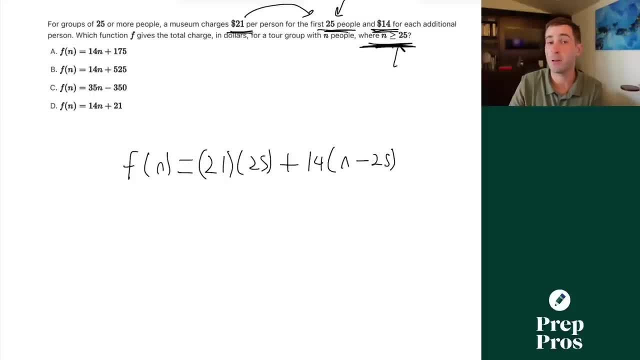 whatever the number of people was in the first group, because we don't want to start double counting those people. They were being charged $21 for the first 25 people, but we need to take away any double charges that we could have otherwise. So here we're going to end up with. f of n is equal to 525 plus 14n minus. 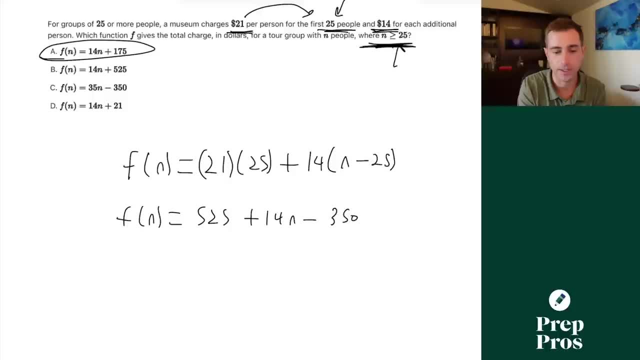 350, and that will leave us with our correct answer of a. Now, if you get to test day and you get to this and you're like, oh, I watched that video but I can't remember how to solve it, this is a great place where you can use a test trick that I call back: solving with points. 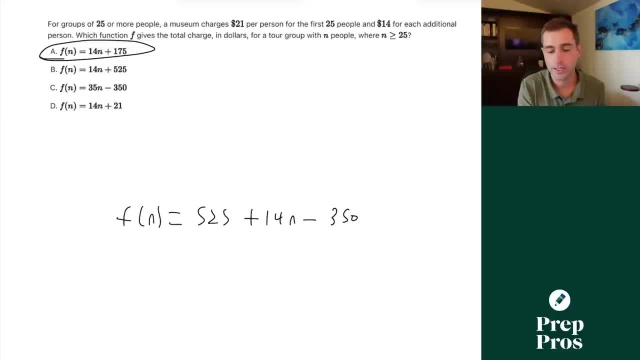 You're simply going to pick a point that you know is true. so let's just say we're going to do it, for what I would do is just the simplest one: 26 people. So if we're going to do it for 26 people, we know our total charge is going to be 25. 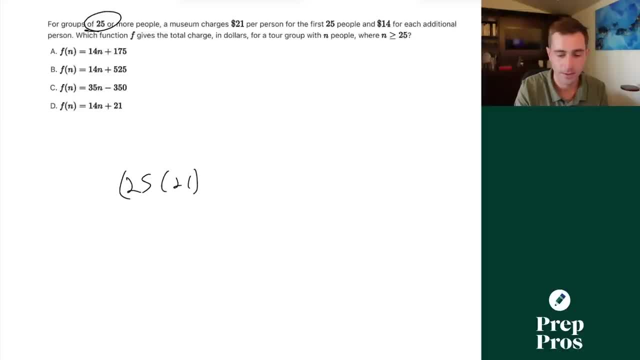 times our 21. get rid of my random little mark there. 25 times 21 plus 14 for the 26 person. This is our first 25 people. this is our 26 person, so this is going to give us a total of 539.. 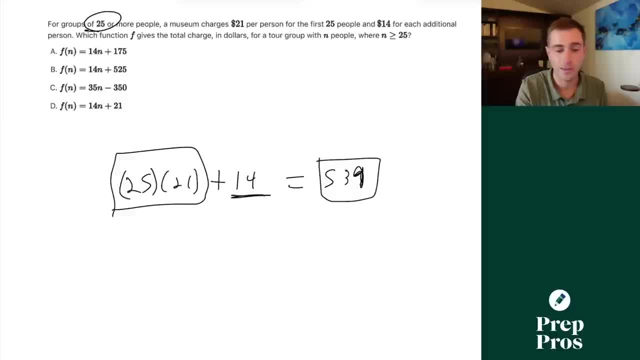 Now all you have to do is use your answer choices and if you plug in 26 for f, for n, excuse me, and the correct answer is going to equal 539.. You're just playing a matching game with these that you know are true gives you a really easy workaround if you blank on the setup on test day. 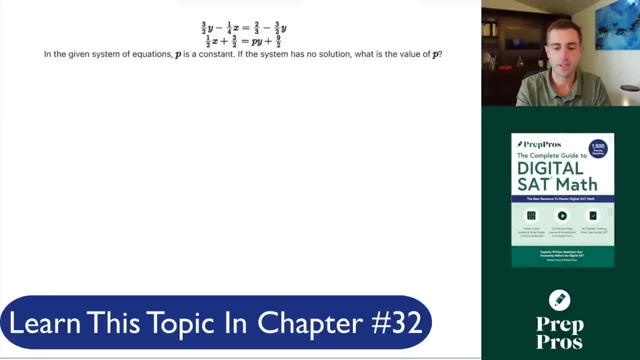 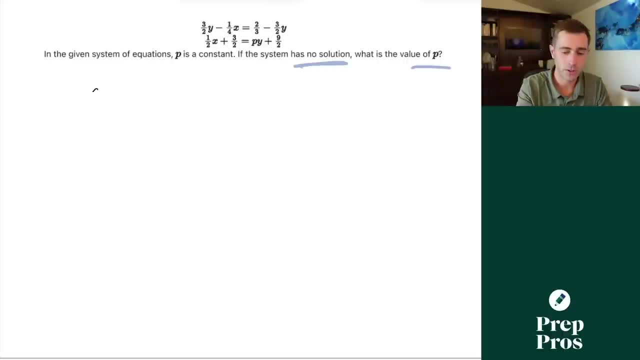 In the given system of equations, p is a constant. if the system has no solution, what is the value of p? Well, what we need to understand here is: systems of equations are really just lines written in standard form: ax plus by equals c. If they have no solution, they have the exact same. 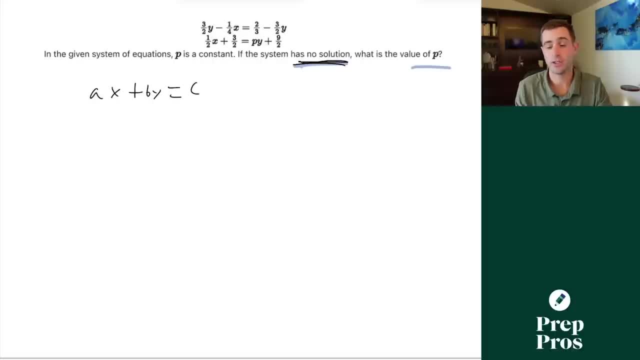 slope, but they have different intercepts. therefore they're never going to intersect each other, never. Now, when stuff is in this standard form, you can always identify the slope by negative a over b. the reason this works is, if we were to solve to put this in: y equals mx plus b form, we'd subtract over. 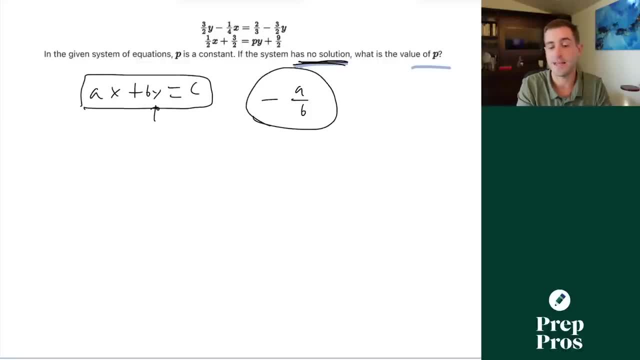 the ax divide by b. that would give us our slope of negative a over b. so i'm just going to go through that to make sure i didn't lose anybody there. so we'd have our by equals negative ax plus c. divide everything by b. that's how we're getting our negative a over b. so this gives us a shortcut that can. 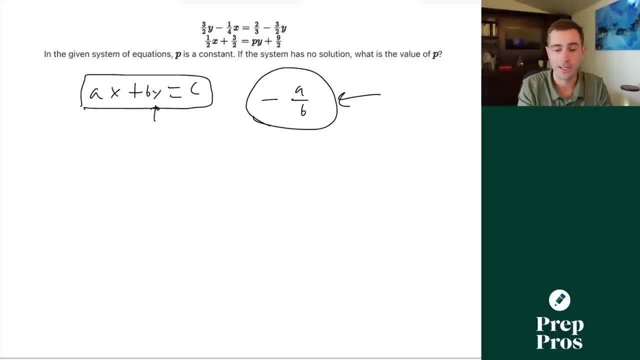 make this question far easier if we know this little trick: instead of having to put these all in y equals mx plus b form, and most likely making a mistake, we just need to put these in ax plus by equals c form and know that negative a over b will give us the slopes. so i'm going to add over my 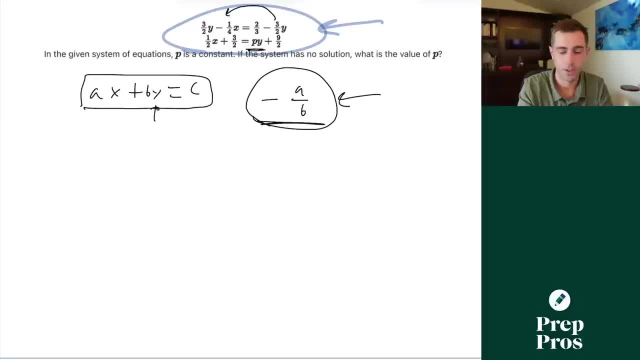 three halves y and i'm going to subtract over my py. so this will end up giving us six halves y, which is also just the same as three y minus one quarter x equals two thirds, and on our bottom equation we'll be left with one half x minus py. i would subtract. 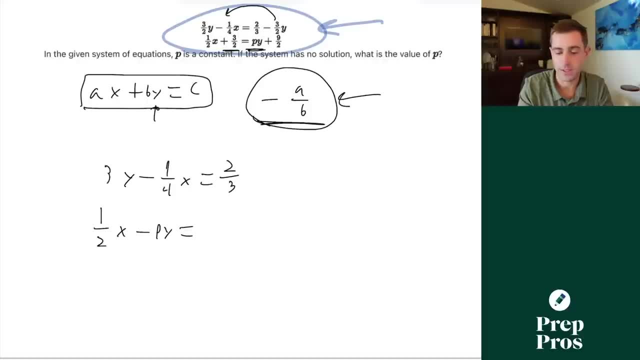 over my three halves. so that is going to give us is equal to six over two, or also just is equal to three here now. this is why the sat has intentionally reordered these is to hopefully lead students into making a mistake if they're going to take this shortcut. so we need to reorder it in ax. 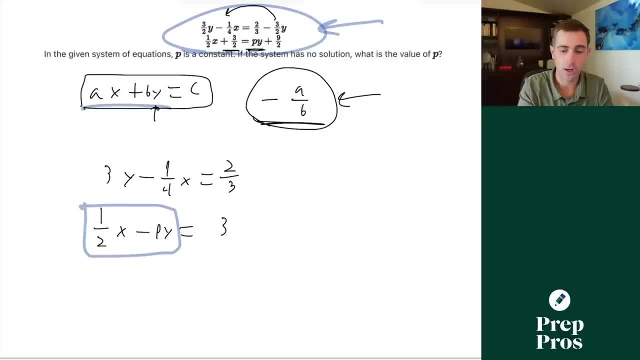 equals c form, which means we need to flip the order of our first portion here. so we're going to go ahead and do that. we're going to go ahead and rewrite this as negative. one quarter x plus three y is equal to two thirds. now what we know is negative. a over b gives us the slope, so negative. 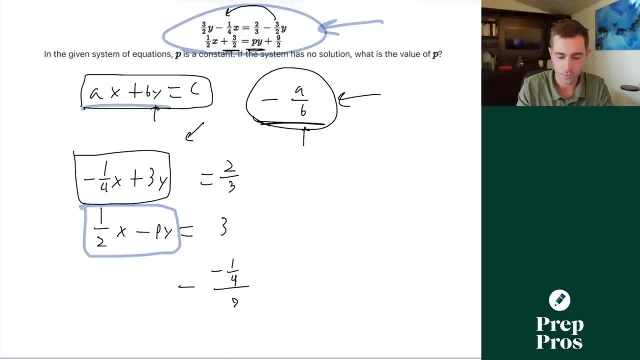 negative one quarter over three is equal to negative one half over negative p. now when i teach this in my book, i just teach this a over b, because the negatives will always cancel each other's out, like we just did now. from here, we just have to cross, multiply and solve through. so we're going to cross multiply. 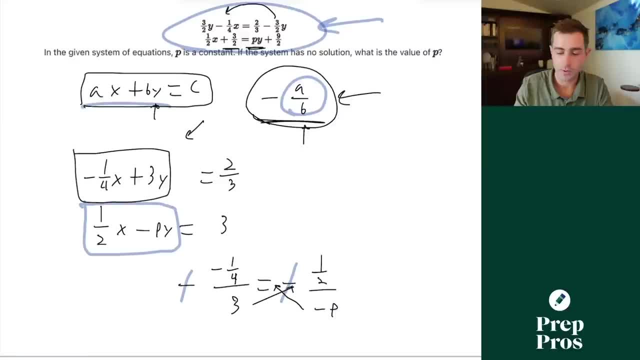 with our p and our three here and as we do that, i'm gonna be left with one quarter. p is equal to three halves. divide both sides by one quarter and that will give me that p is equal to six, and that will give me the right answer. 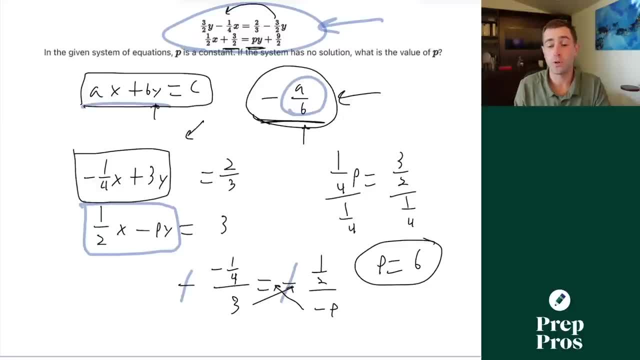 So if you learn this trick, you're able to really start going through these questions that are supposed to be one of the last questions of the test very, very quickly and efficiently, and it cuts out a ton of mistakes that you normally would make. 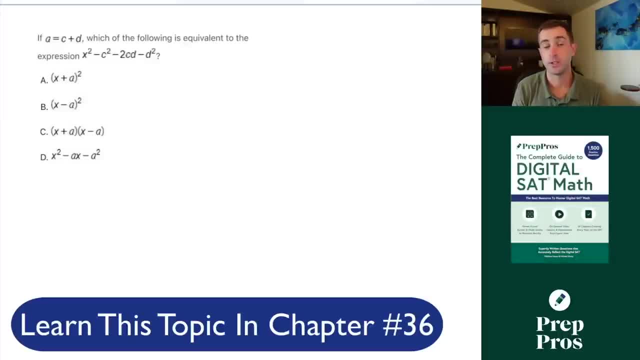 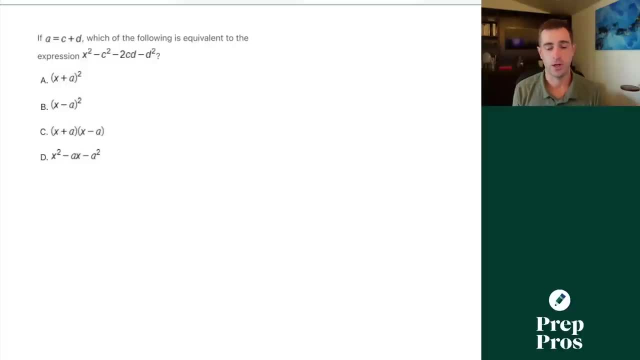 If a equals c plus d, which of the following is equivalent to the expression x squared minus c squared minus 2cd minus d squared? This stumps almost every student on the test, and we're going to go through the technical way, and then I'm going to blow your mind. 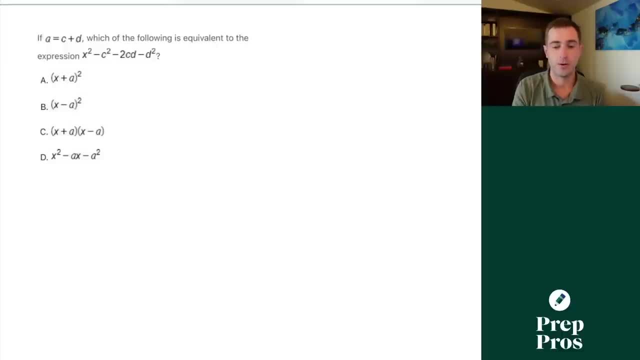 with how we can actually use Desmos to solve this as well. Now, if you see questions like this, it's almost always what I call a special quadratics question, and this is around your perfect squares of addition, subtraction or difference of squares. 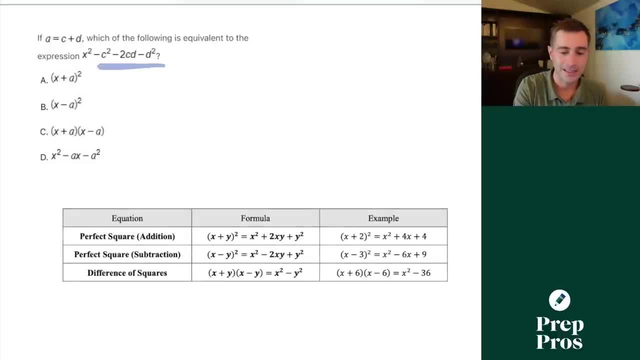 So I'm always looking for those patterns and what I notice is: this is really going to be our perfect squares of addition, but we're going to have to be subtracting this entire expression as we go through, because if we do, c plus d squared. 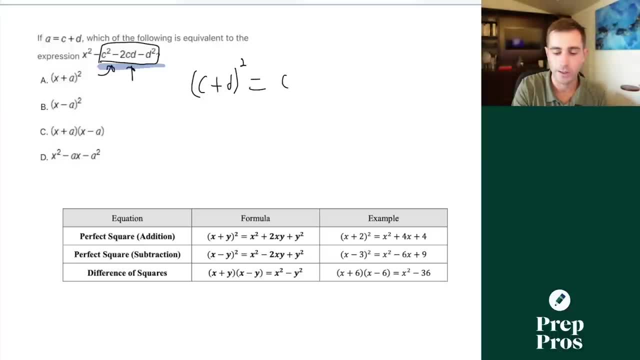 the same way we would do x plus y squared. that's going to get us our c squared plus d squared, minus 2cd, minus 2cd plus 2cd plus d squared. Now, if we want to have all of this negative, 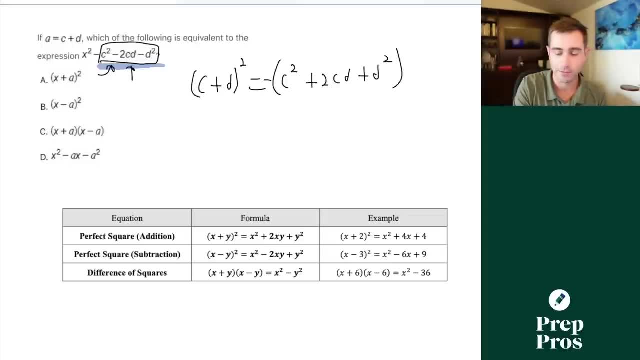 we simply just need to basically distribute a negative through this entire portion. So we want to be doing x squared minus if we know that a is equal to c plus d. we want to be doing x squared minus a squared because, since we know a is equal to c plus d, 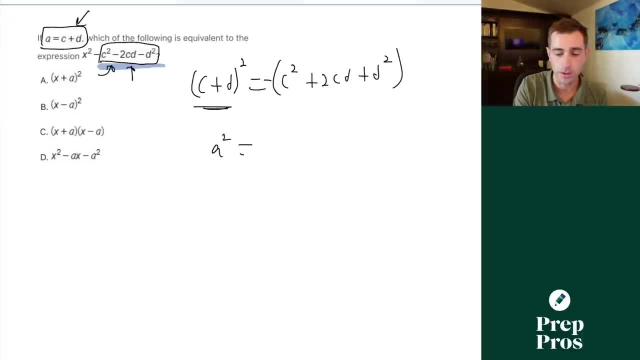 c plus d squared is also the same as a squared, so a squared Also. we'll get rid of that negative that I added in as we were talking through. a squared is also going to equal this same c squared plus 2cd plus d squared. 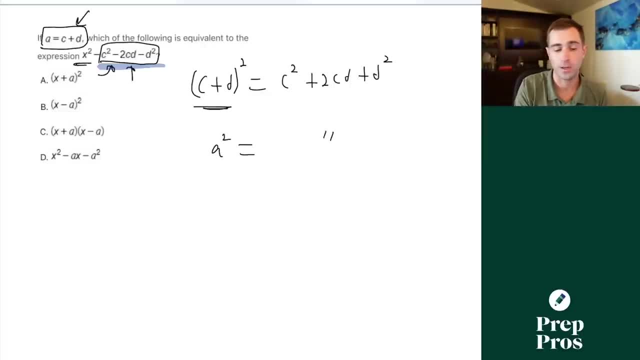 so we just want to get x squared minus a squared, and x plus a times x minus a is going to get us there. That's our difference of squares. That's going to give us x squared minus a squared. x times x gives us our x squared. 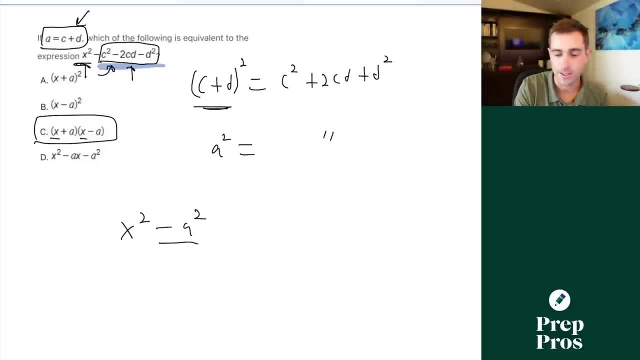 We know negative a squared is going to give us negative of this entire expression and that will give us our minus c squared, minus 2cd, minus d squared- Really, really hard to spot. So let's jump over to Desmos and go through a hack. 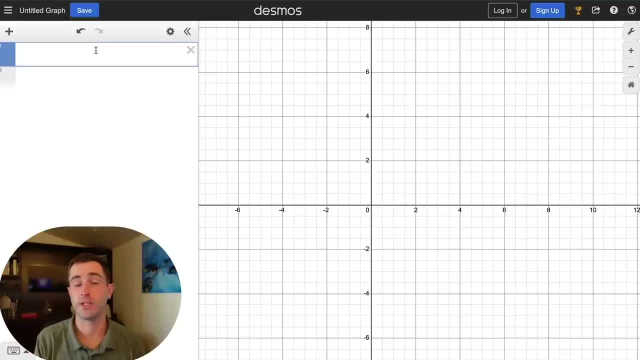 Now, this is actually one of my favorite Desmos hacks. It's just a bit of a trickier version of this, and this is what I call the equivalent hack. If things are equivalent, they're graphically the same, So we just need to start breaking all this stuff down. 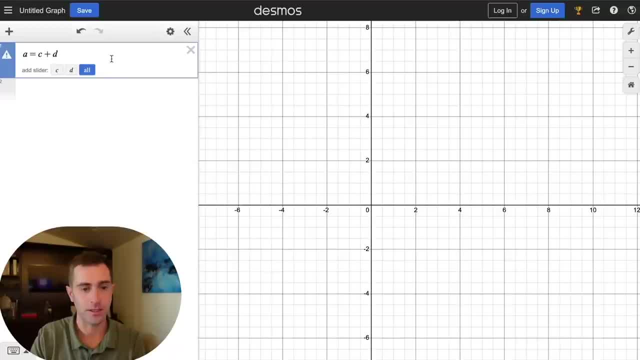 What we know is we were told that a equals c plus d. Now we're going to have to click add a slider. This is going to just put in values for us. We're going to set the values to will not affect this question. 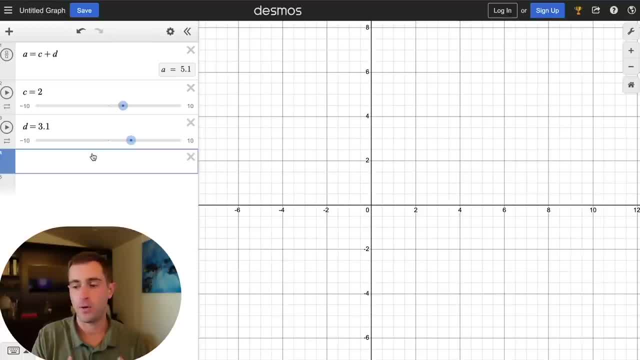 I recommend just going through this and getting used to some of this yourself. Now, what we know is: a equals c plus d. We're looking for which of the following is equivalent to the expression. I always graph these as: y equals x to the second, minus rc to the second. 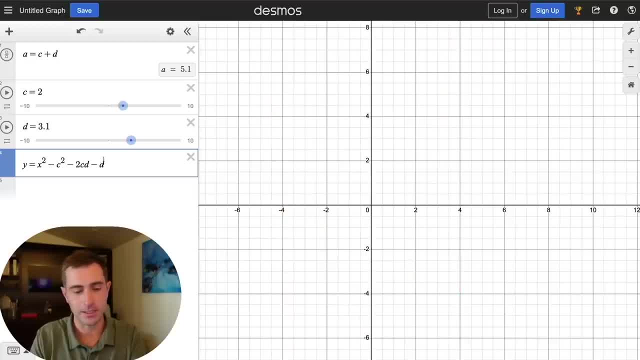 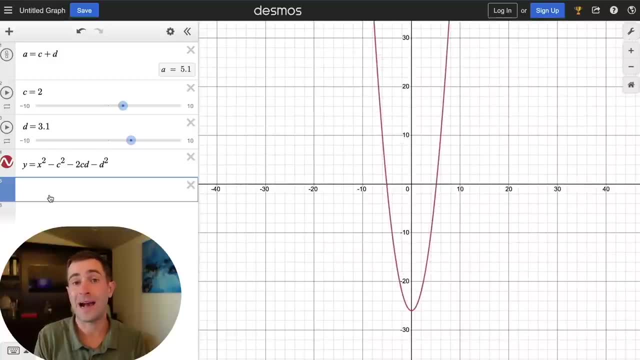 minus r2cd, minus d to the second. So this is going to give us this graph, So we'll zoom on out, so we get the graph there. Now, if things are equivalent, they're graphically the same. In other words, they're identical. 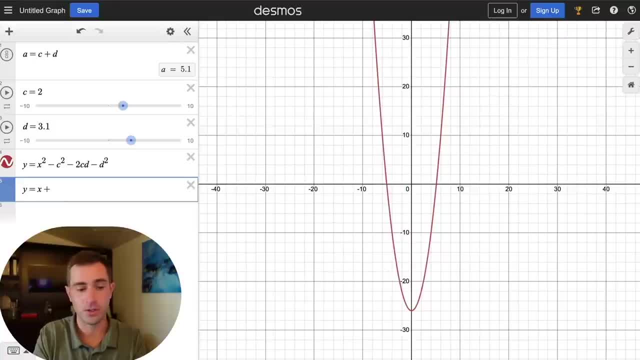 So we can just also see that c is our correct answer, because if we do y equals x plus a, times x minus a, we get the exact same graph. Now we can always tell stuff is equivalent. You turn the graph on and off. 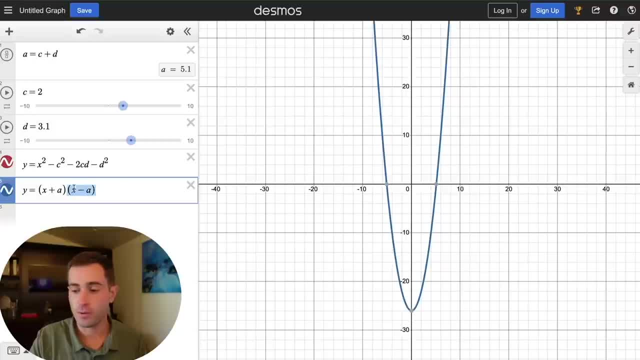 It gives you the exact same graph that tells you it's right. Now. if we were to try to check a- not the same graph. If we were to try to check b- not the same graph. And if we were to go through, 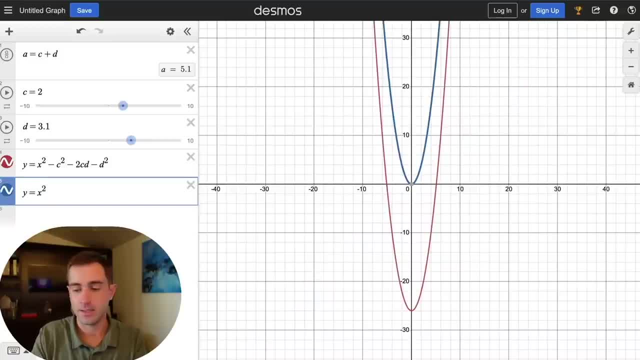 and check d. as you will see, this is an amazing hack for the test. Doesn't give us minus a squared, not x squared, excuse me, doesn't give us the same graph. So this is one of the key Desmos hacks that I teach in my book. 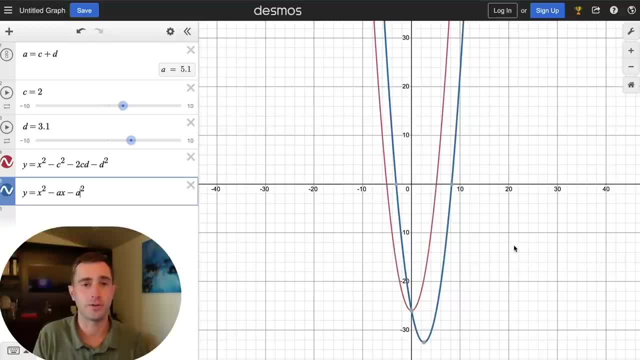 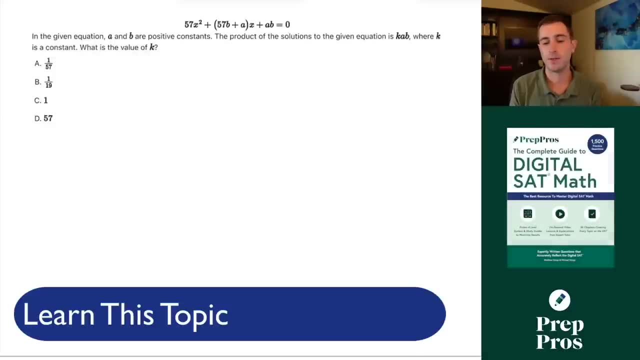 I'm going to put together an entire Desmos course shortly to go through all the different ways you can take advantage of it for some of these really creative, challenging questions. and all the basics In the given equation, a and b are positive constants. 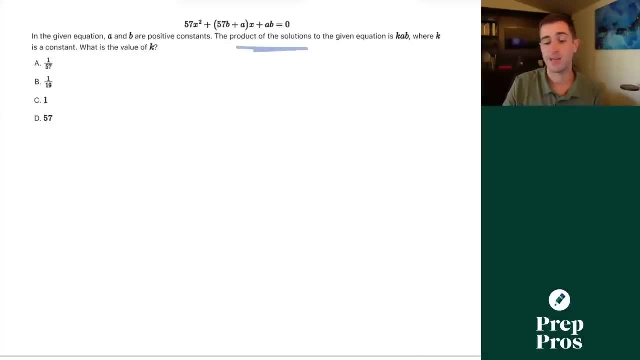 The product of the solutions to the given equation is k a b, where k is a constant. What is the value of k? This is just specific knowledge. Your product of solutions for any quadratic in ax squared plus bx plus c form is always just c over a. 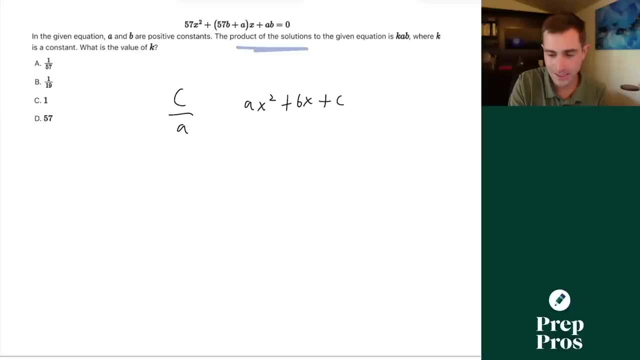 So that ax squared plus bx plus c, whenever it's equal to zero or equal to y, just c over a. So our a value here is 57.. Our c value is ab. So we know ab over 57 is the product of our solutions. 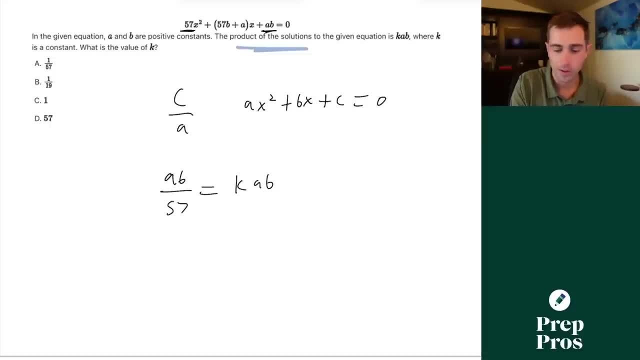 This is equal to k- ab. Well, we can divide both sides by ab. That's going to cancel out the ab's. That's going to leave us with 1 over 57 is equal to k. We're able to find our right answer pretty easily. 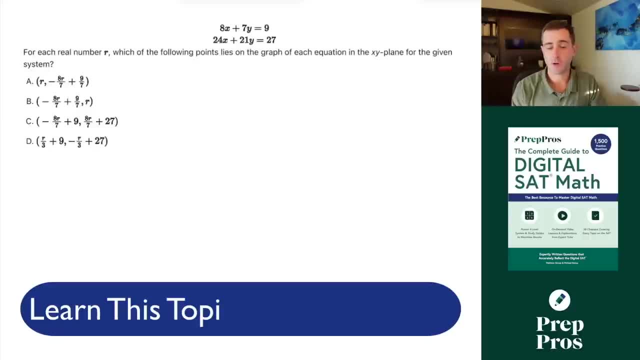 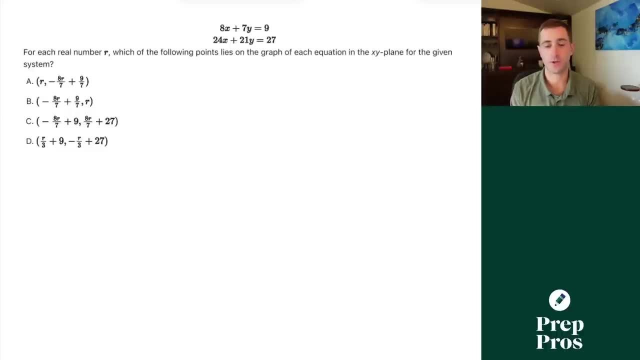 if we just know that correct knowledge For each real number r, which of the following points lies on the graph of the equation in the xy plane for the given system. Now, one thing we know here is if we plug in our x and y values. 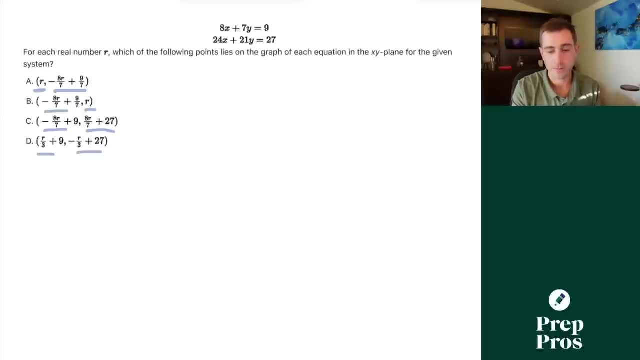 as we go through each of these. if both sides of these equations are equal, that tells us. the point lies on that graph as we're going through Now. we can go through and we could just manually plug in all of these and we're eventually going to find the right answer. 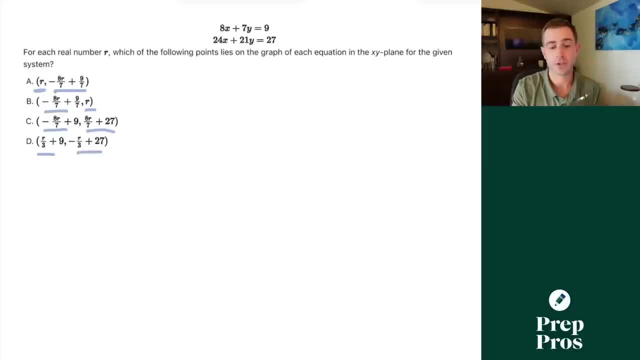 as long as we understand that principle, which means this question isn't nearly as awful as it looks, But we want to be able to identify the right answer really quickly because time is so important on test day. So there's a pattern that comes up with this type of question. 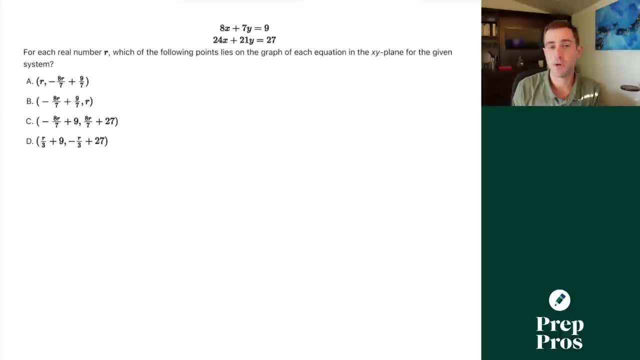 that lets you jump and find the right answer really quickly. Since everything has to be equivalent, we have to start canceling stuff out. So what I mean by that is I can immediately tell that a is going to be my right answer, and we'll just start by looking at our first one. 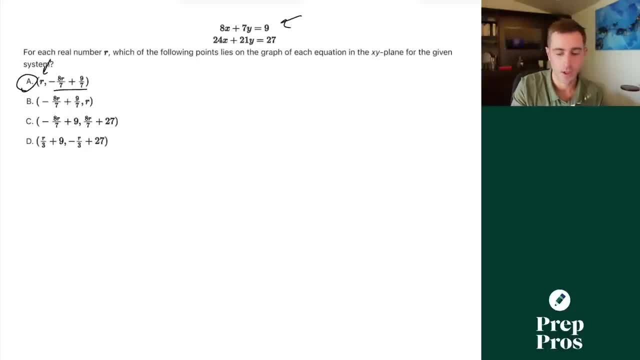 So when we plug this in, here's our x value, here's our y value. So we're going to get 8r. Pretty easy to figure that out: 8 times x, we're plugging in r for x. So what I'm looking for as I'm looking through each of these answer choices: 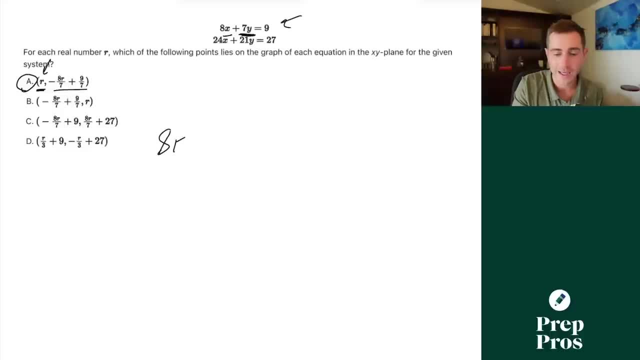 is canceling everything out. So what I'm doing for y is going to have to cancel out that 8r I just created and make it equal to 9.. And that's how I can see this negative 8r over 7,. 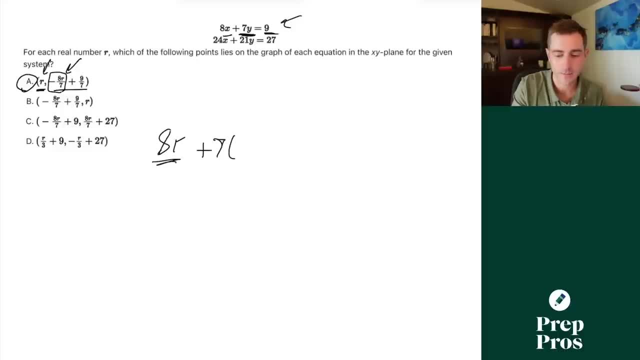 well, plus 7 times, I'll clean up my 7 there. negative 8r over 7, well, 7 and 7 cancel out. 8r negative 8r cancel out. So we're good there. 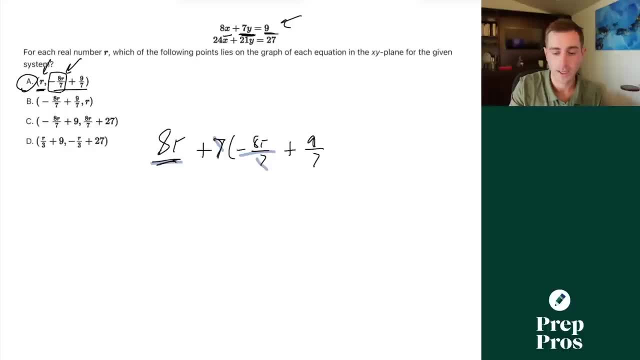 Plus our 9 over 7, once again, our 7 and 7 cancel out, and now we're going to be left with that. 9 is equal to 9 as we go through. So what happens here? we'll write it all out. 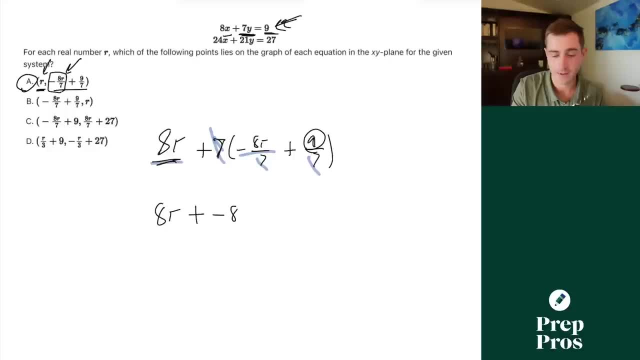 but 8r, we're going to get plus negative. 8r plus 9 is equal to 9.. These cancel out. That's how I can find my right answer very quickly. The exact same thing happens when we check our bottom equation. 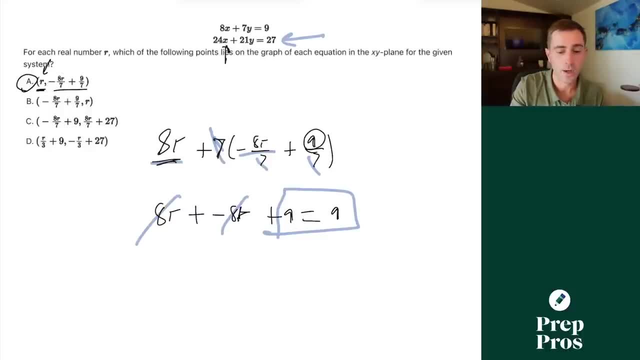 We'll get our 24r. Well, 21 times negative 8 sevenths is going to give us negative 24, so we're going to create a negative 24r. 21 times 9 sevenths is going to equal 27,. 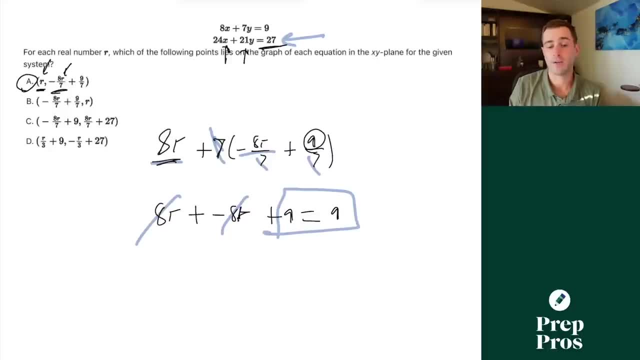 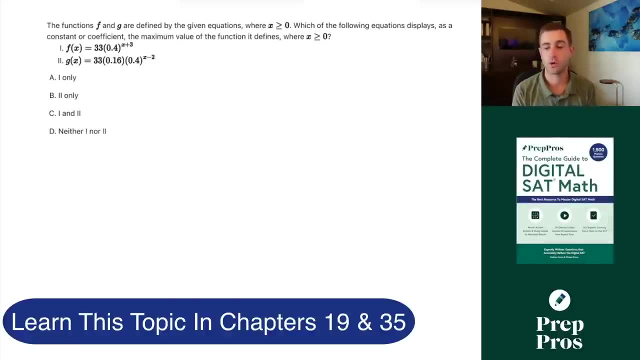 and that's how we can spot our right answer very quickly and efficiently for this type of question. The functions f and g are defined by the given equations, where x is greater than or equal to 0.. Which of the following equations displays as a constant or coefficient: 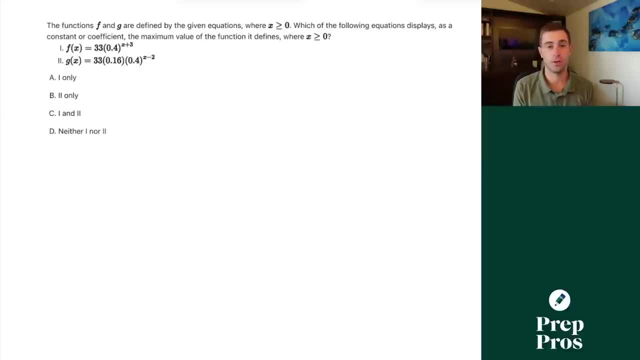 the maximum value of the function. it defines where x is greater than or equal to 0?. Most students just look at this and have no idea where to start, but we're going to make sure you feel really comfortable with all of this Now. the first thing we need to understand is the basics of exponential growth and decay. 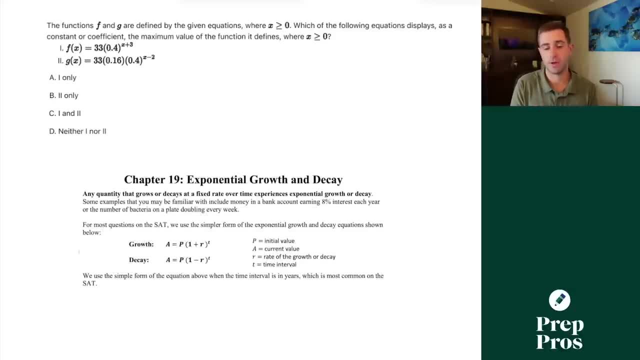 So I'm going to pop on the screen a little bit of info from my book here for the basics. but what we need to understand is this is our starting value. this is going to be showing us our increase or decrease and this is going to be dealing with our powers here. 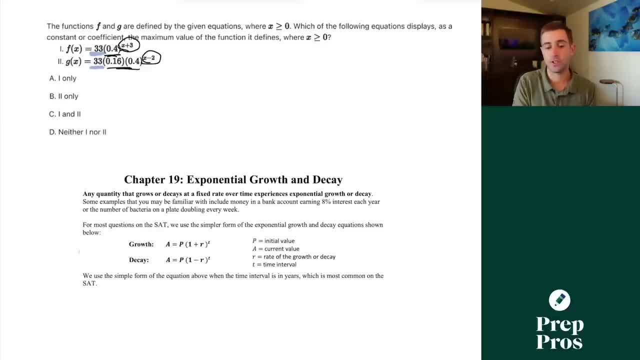 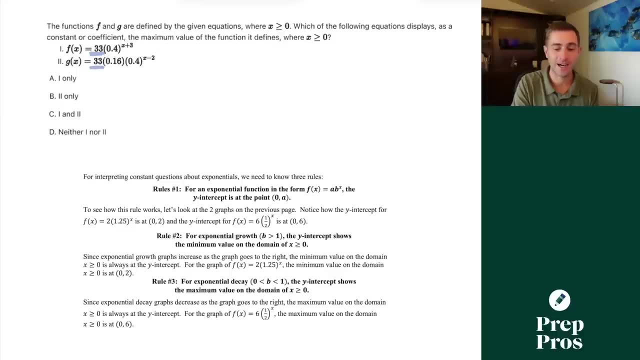 But if we're saying the constant or coefficient is a maximum value, I'm going to pop on some rules from another chapter. now. This is how complex of a question this is. The constant showing a maximum is going to have to be showing that 33 is our y-intercept. 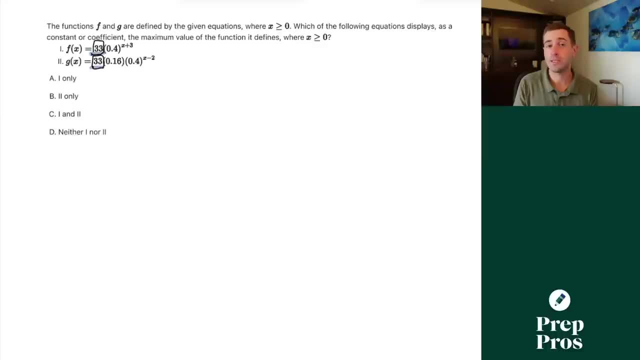 And this is why we're going to jump over to Desmos in a minute, and Desmos really is the simplest way that we can solve this, Once we understand and we decode all that information. well, if the y-intercept is the greatest value on the graph and it equals 33,, 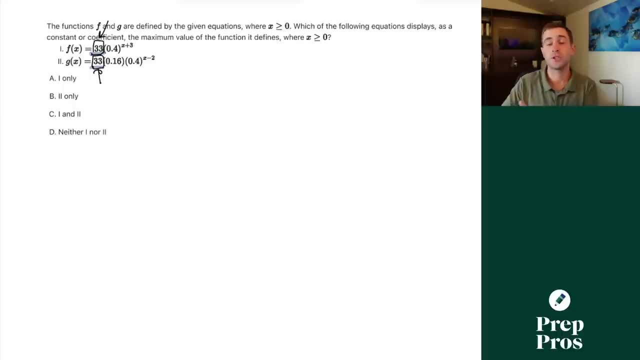 that's going to let us see. if this question is correct, We can take this super complex question and make it far easier. Now we're still going to go through the technical way because it actually teaches some really important exponent skills and lets you see how difficult some of these questions are. 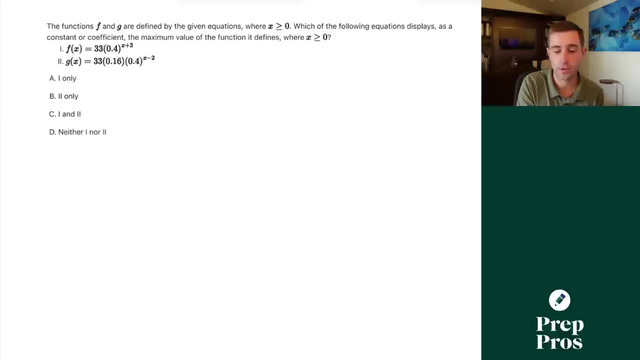 until you understand the Desmos way of doing it. So, as we said, what we're looking for is seeing if the y-intercept is actually 33.. Now for both of these. since it's a maximum, it needs to be a decreasing exponential function. 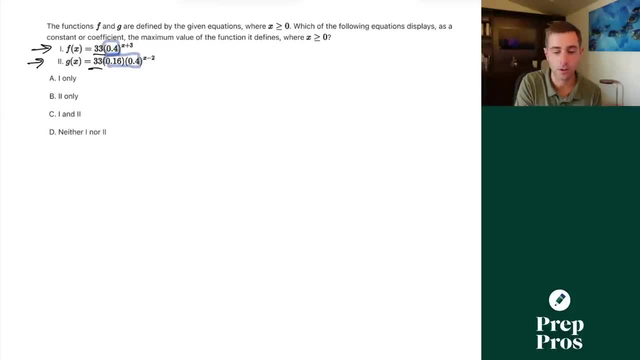 If it's less than 1, this is going to be decreasing. So it looks like on first glance and where the SAT tricks students is. a lot of students look at this and they go: ooh, both of these work, They both have 33 and they're decreasing. 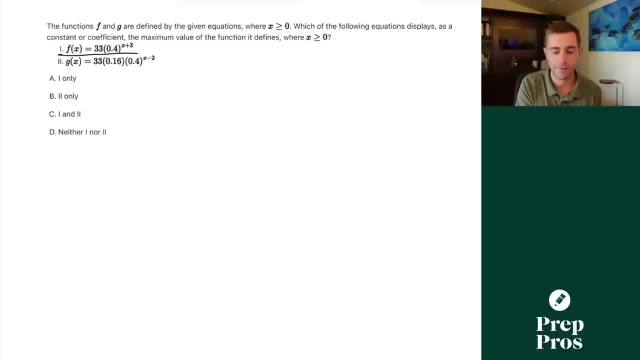 but we have something a little sneaky that they're doing with the exponents. So if we take our f of x, we can actually expand this out by writing this as: f of x equals 33 times 0.4 to the x times 0.4 to the third. 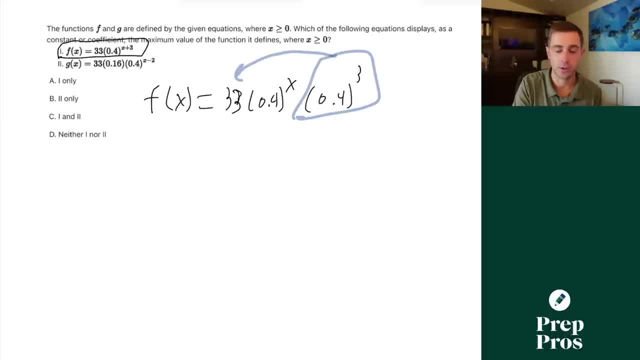 And this 0.4 to the third when it gets distributed back to our 33, because if we're simplifying this, we're going to rewrite this as f of x equals 33 times 0.4 to the third, times our 0.4 to the x. 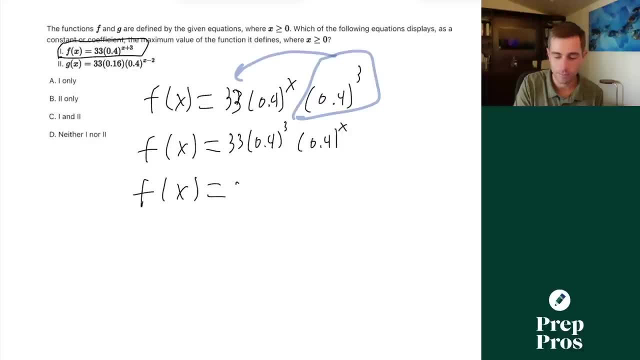 Well, this is going to give us something loosely about 2.1 times 0.4 to the x And going back to our exponential growth and decay, this would be saying our graph is starting at 2.1 and it's showing decrease every unit of x after. 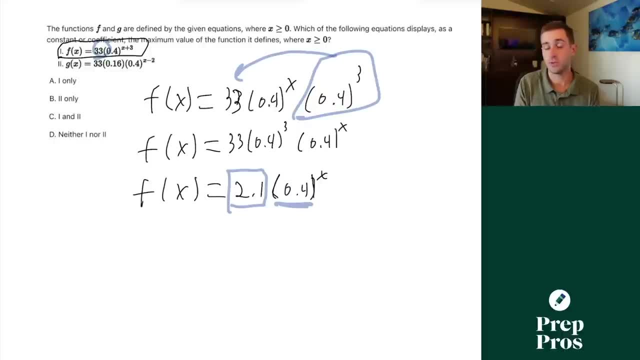 But that doesn't show us 33 in this original form, so that does not display as a constant or coefficient the maximum of the function. So 1 doesn't work Now as we get to 2, once again we have some tricky exponent stuff. 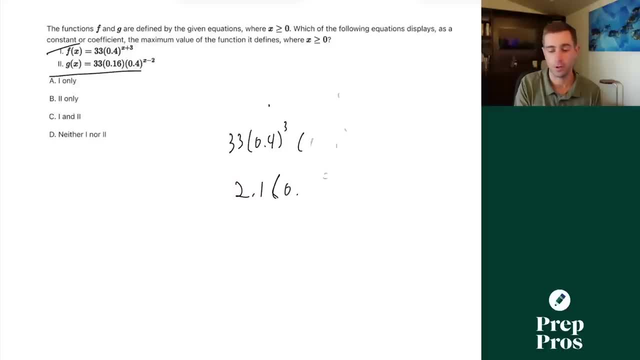 but this one ends up working because we're going to cancel something out perfectly here. Now, as we work through this, we have to expand this back out, So we're going to rewrite this once again as: g of x equals 33 times 0.16. 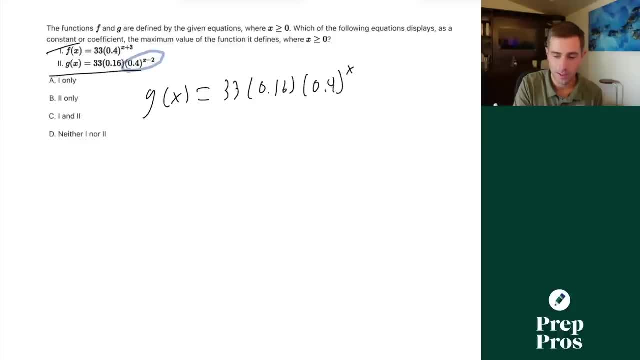 times 0.4 to the x times 0.4 to the negative second. Now this is going to be the same as g of x equals 33 times 0.16 times 0.4 to the negative second is the same as 1 over 0.4 squared. 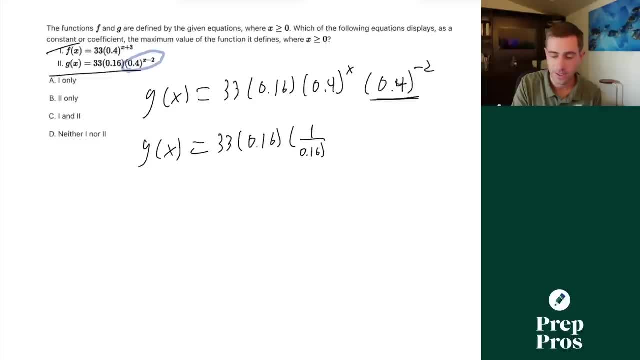 which is the same as 1 over 0.16.. Put this entire thing in parentheses here. Go back and clean that up so nobody gets confused, And then we'll have our same 0.4 to the x. Now these are going to cancel out. 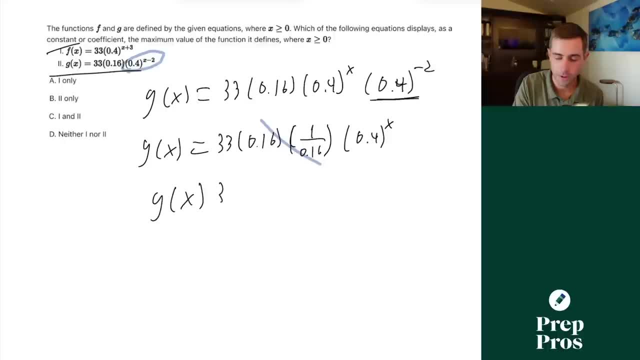 and this is going to give us our form of 33. g of x equals 33 times 0.4 to the x. So this does show us our y-intercept. our maximum value is 33, and it's decreasing by 60% every single time. 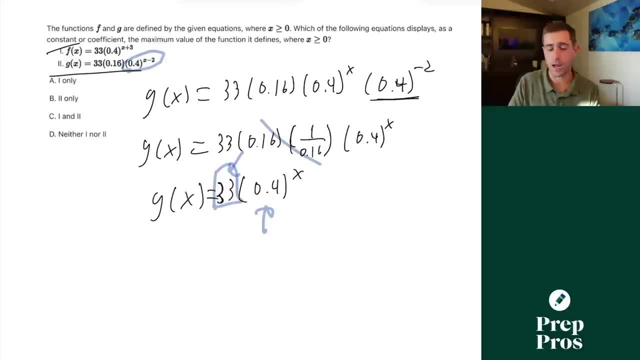 So we're going to have a single increase of x as we go through of the prior term. That's why only two works. Now, this is an incredibly difficult question. So, as I said, we're going to jump over to Desmos, And if that felt a little tricky, 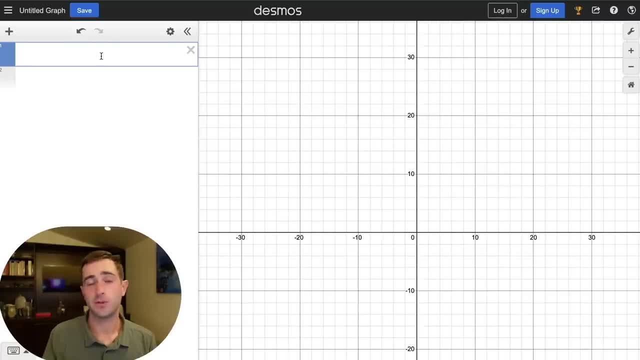 I promise it's going to clear up a lot more as we go there. Now we can actually use Desmos to solve this question, but we do still need to understand the underlying concept. And here, since we're looking for that maximum, we're looking to see 33 as our y-intercept. 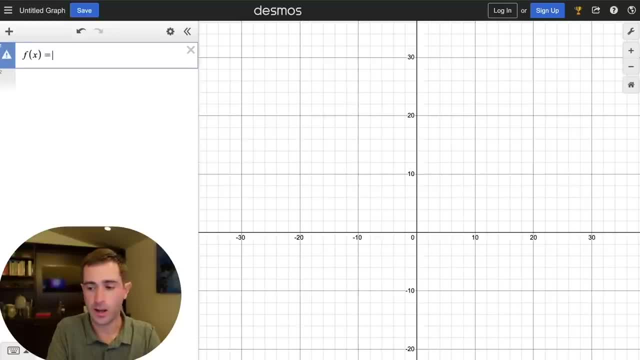 So we can just graph this And if we see 33 as our y-intercept, that's going to tell us that we found the right answer. So that's one of the things that we need to know about Desmos to graph this properly. 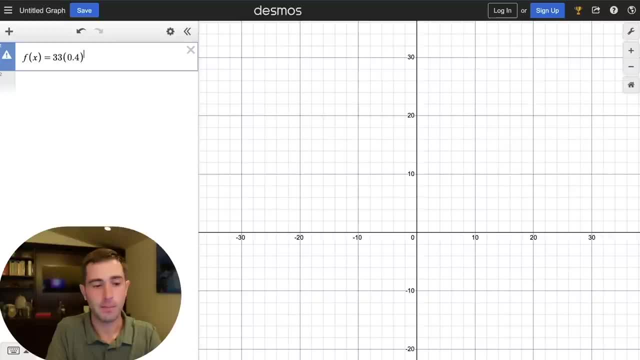 Now you're going to use that little caret button, which is above 6 on most laptops, But if we just try to enter an x plus 3, Desmos isn't going to cooperate, So you're going to have to do parentheses: x plus 3.. 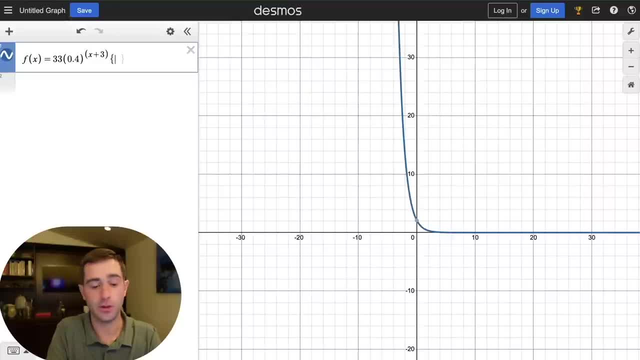 And then we want to set up a restriction where x is greater than or equal to 0. So we're going to use our curly bars and do: x is greater than or equal to 0. Close our curly bars. Looks like my mental math was pretty good. 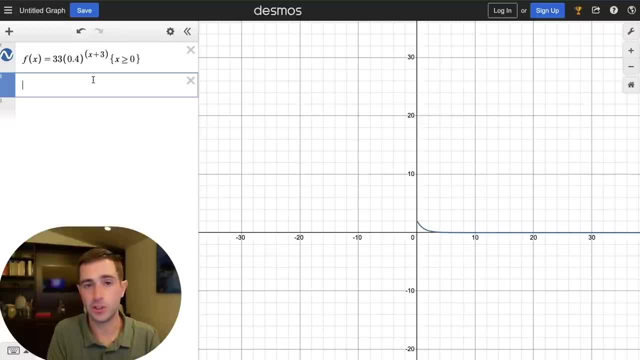 We got that y-intercept of about 2.1.. Doesn't show us the maximum is a constant or coefficient. So now we'll go over to g of x. Now, as we do that same exact thing, We can simply enter this in: 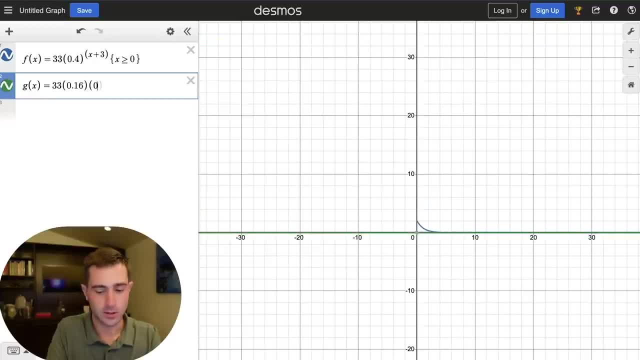 33 times our 0.16 times our 0.42.. Once again, use your parentheses, Our x minus 2.. And when we do that we'll finish with our curly bars. but you can kind of already see the correct answer here. 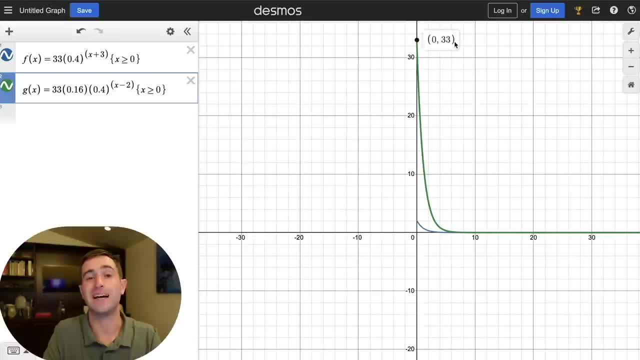 This gives us that y-intercept of 33 that we're looking for. That shows us the maximum is our constant or coefficient. Desmos can really really help you out, but you still need to learn the underlying concepts. That's why I always try to integrate Desmos chapter by chapter. 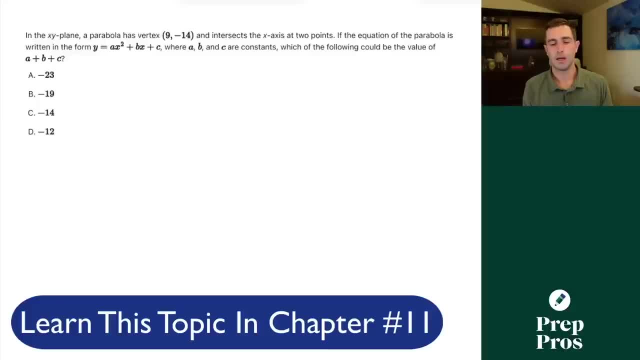 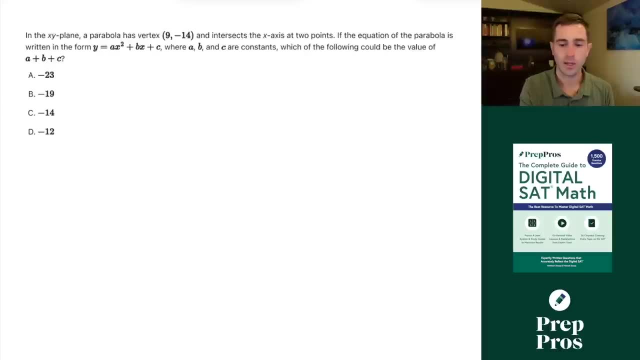 on how you can apply it in my math course. In the xy-plane, a parabola has vertex 9, negative 14 and intersects the x-axis at two points. So since my y value is negative, this tells me it's an upwards-facing parabola. 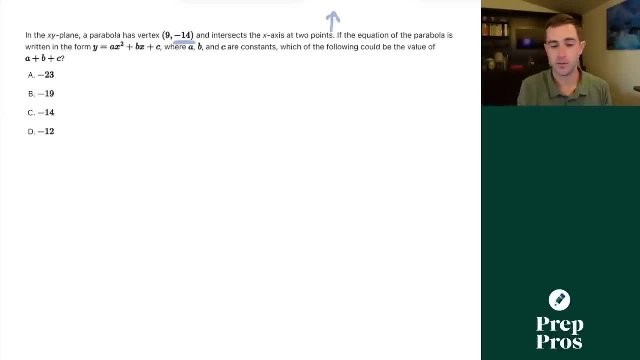 If the equation of the parabola is written in the form: y equals ax squared plus bx plus c, where a, b and c are constants, which of the following could be the value of a plus b plus c? Well, I can't immediately get to a plus b plus c form. 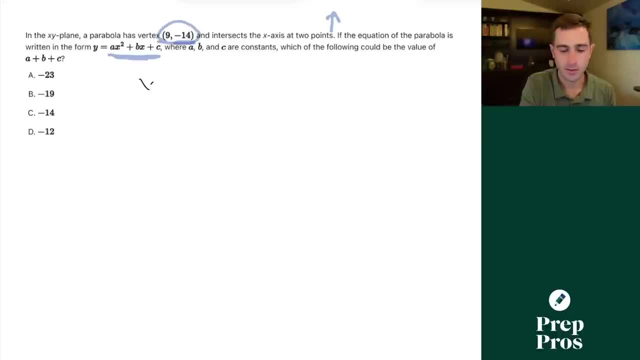 but I can use vertex form to get me there Now. our vertex form is: y equals a times our x minus h squared, plus k. h is our x-coordinate of the vertex. so this is going to be x minus 9 squared, and this is our a over here. 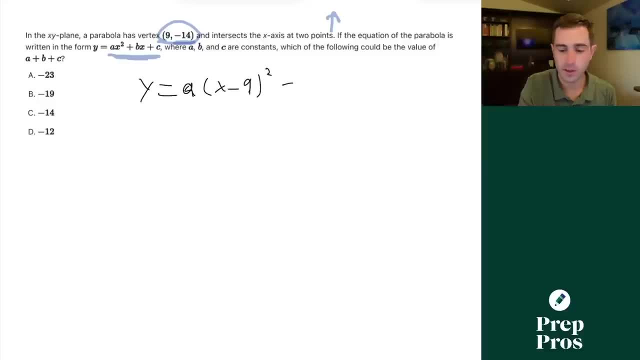 And plus k. well, that's negative 14, so we'll have minus 14.. So we'll start expanding this out. We'll have y equals a times x squared minus 18x plus 81.. I'm just getting that by foiling out x minus 9 times x minus 9.. 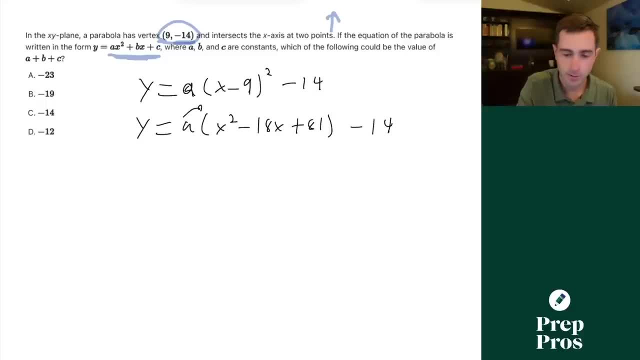 And then we'll have our minus 14.. And now I'm going to distribute the a through all of these terms, So we'll have y equals ax squared minus 18ax plus 81a minus 14.. And we know this is going to be equivalent to: 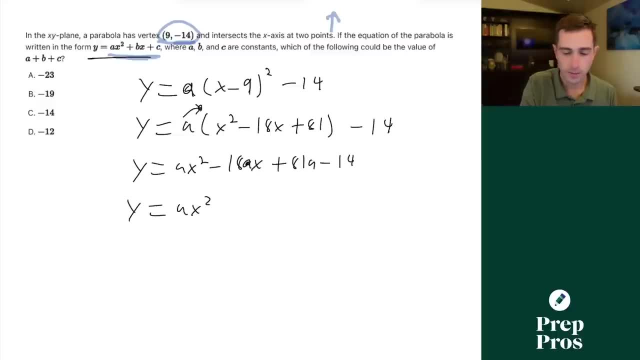 our y equals ax squared plus bx plus c. So what I know is a equals a negative 18a equals b and 81a minus 14 is equal to c. So we'll rewrite those statements: a equals a, b equals negative 18a. 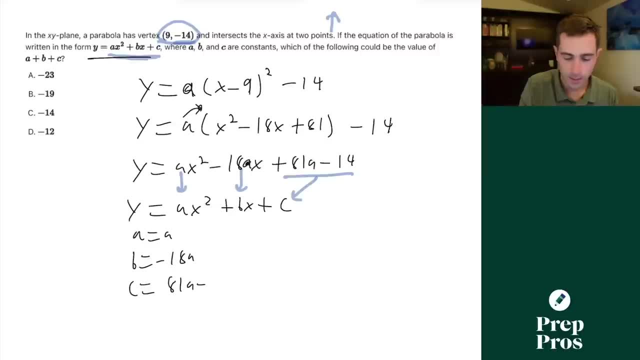 and c is equal to 81a minus 14.. So now we can take this entire a plus b plus c statement. we can just put it in terms of a, so it's easier for us to work through. So that's just going to be well. a is a. 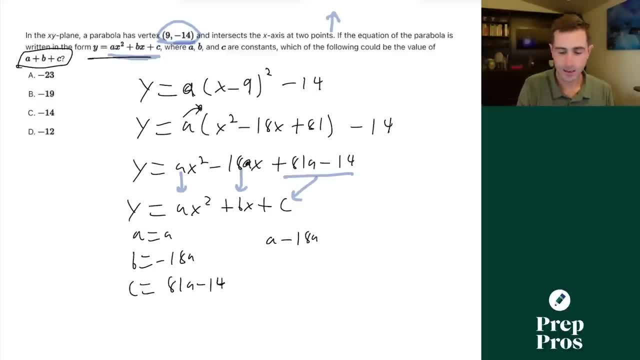 so we're going to do a minus 18a plus our 81a minus 14, and that's going to simplify down to 64a minus 14.. And now it's normal to kind of get a little stumped. We've done all this work correctly. 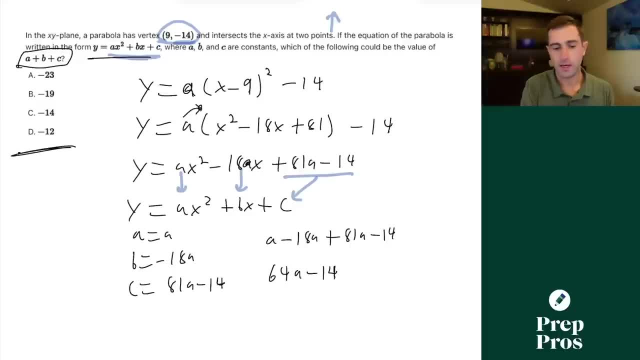 but how are we supposed to figure out which of these could be a value of a plus b plus c? Well, we know, 64a minus 14 is the same as a plus b plus c. and going back to our first sentence, we know, as we talked about, 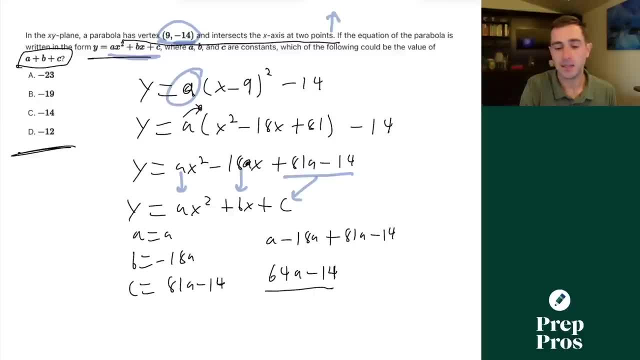 that our a value here has to be positive as we're going through, because our y coordinate is below the x axis and since it's intersecting the x axis at two points, it's an upwards facing parabola, as we talked about earlier. 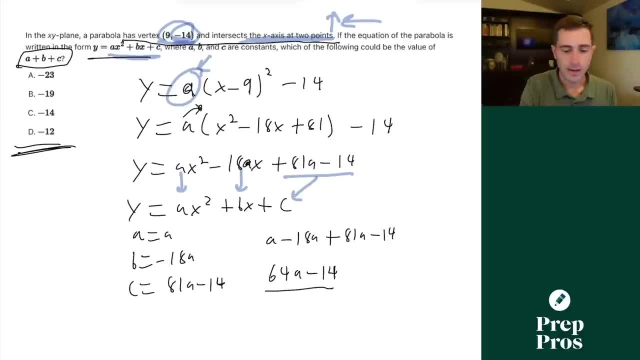 So what we therefore know is whichever of these answer choices is correct, when we set it equal to 64a minus 14, it must give us a positive value, And that's why d is our right answer, because if we do, 64a minus 14 equals negative 12,. 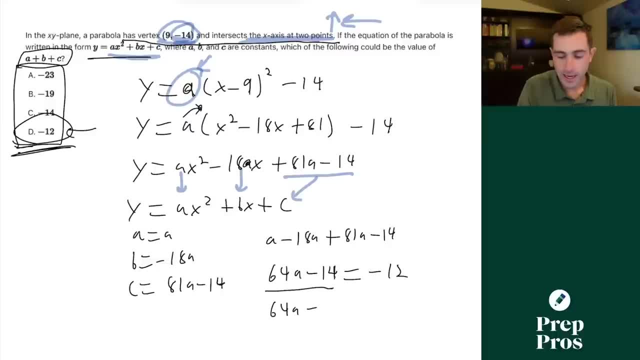 well, we add over the 14, we get that 64a is equal to 2, and that's going to give us that 64a is equal to 1 over 32.. Now, if we plugged in negative 14,, well, negative 14 plus 14,. 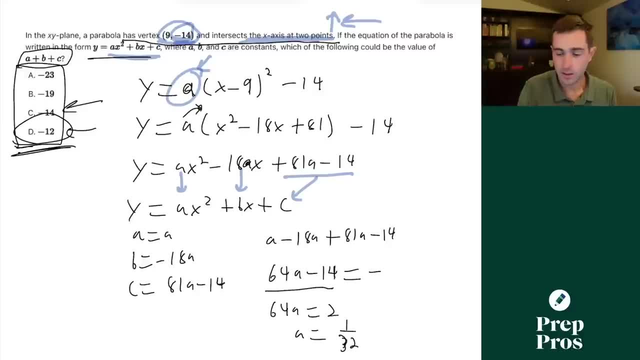 if we pop in our negative 14 over here, well, we would just get: 64a is equal to 0, and that's not going to give us a positive value. and then with the 19 and the negative 20, negative 19 and negative 23,. 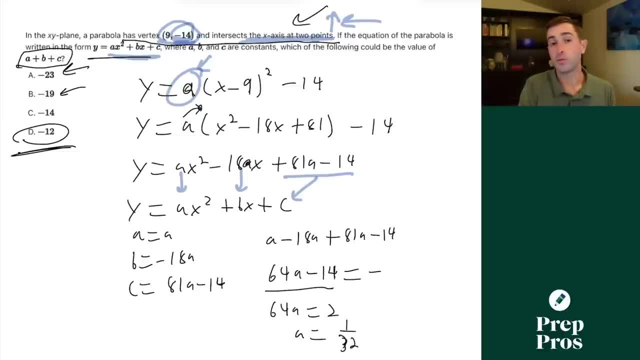 we're going to get negative a values, so we're going to be breaking the rule of that first sentence. This is about as hard of a question as you could ever see on the digital SAT. but if you see really tricky stuff like this, 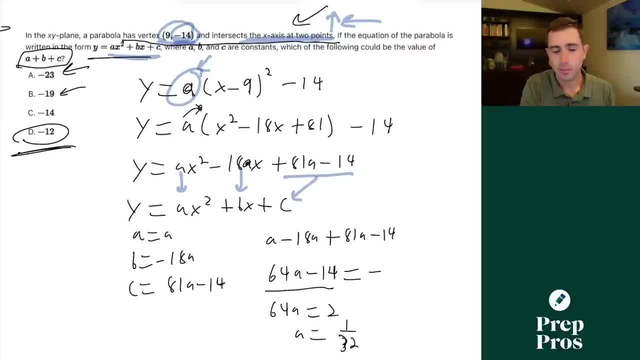 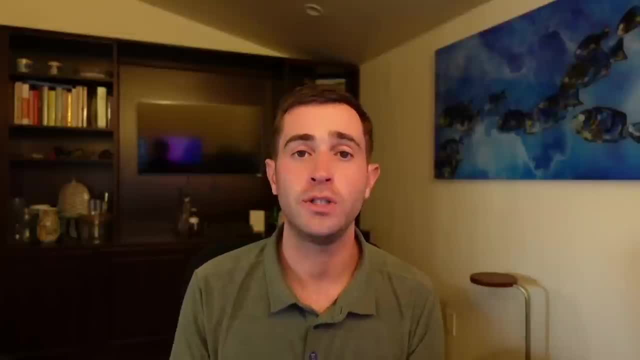 you're probably going to have to reread the question to start picking out little clues that are going to help you know where you should go. I really hope this video helped you out. Now we're going to talk about resources that you can use to better prepare yourself. 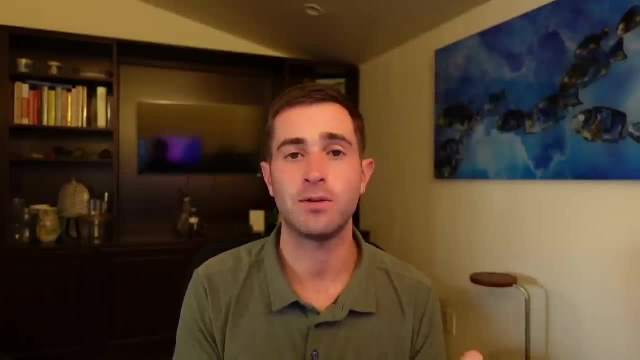 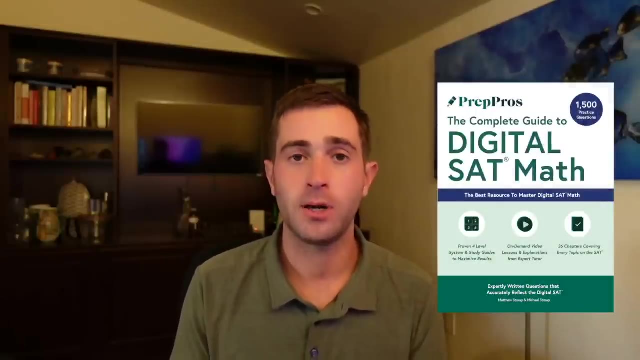 Now, the first thing you may have noticed as we were working through the video is I was popping on the screen where you could learn more about that topic in my new digital SAT math book. So I was popping on the chapter numbers. so if you noticed any topics, 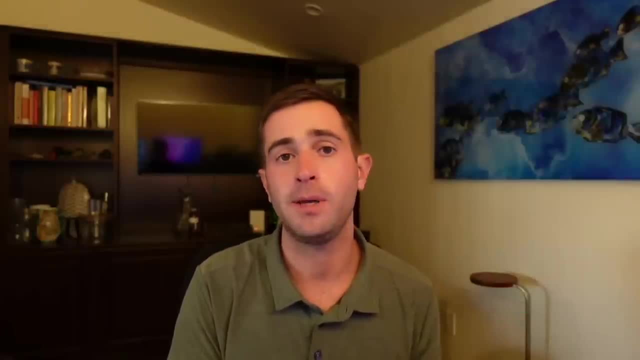 that you wanted more education in or you wanted more practice in. it would be great to pick up a copy and just jump straight into those chapters and then you can start digging into those. We really just kind of scraped the surface for digital SAT math in this video. 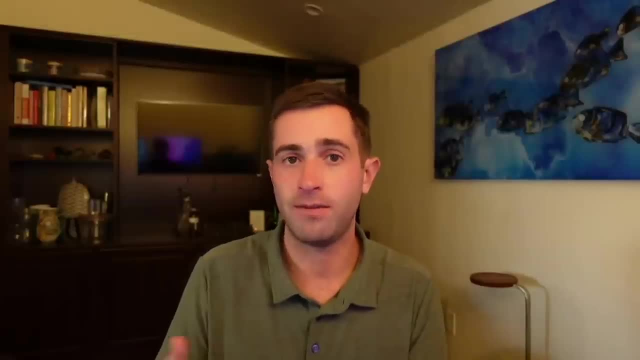 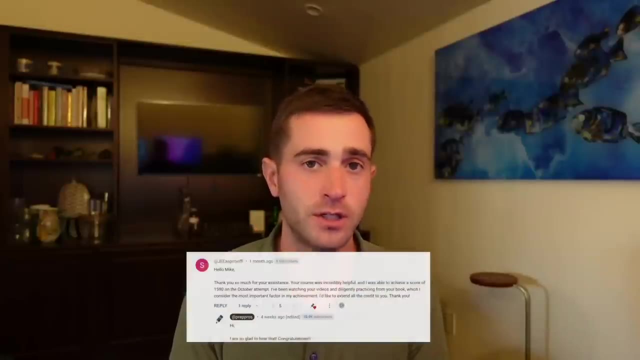 so there's a lot more advanced question types, a lot of tips and tricks and strategies that you need to learn if you want to get a 750 to 800 on the test. Now, the other thing that I would recommend using is my ultimate SAT course. 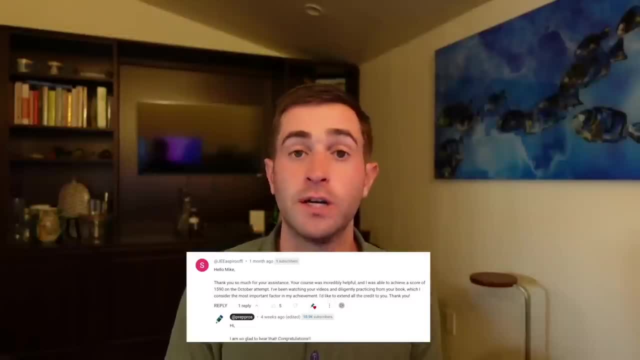 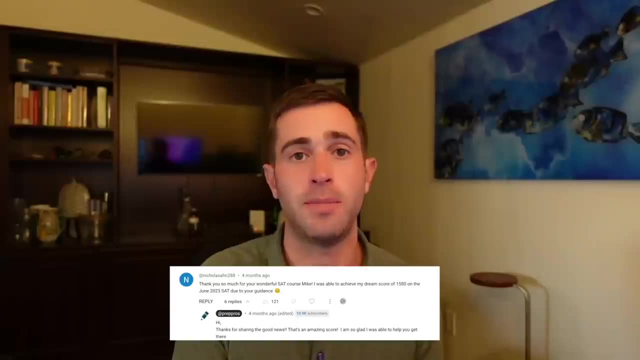 I've just finished completely revamping it for the new digital SAT. It's for international students who've been taking the digital SAT for over a year and it's delivered amazing results for students in the past. I've had well over a thousand students use it. 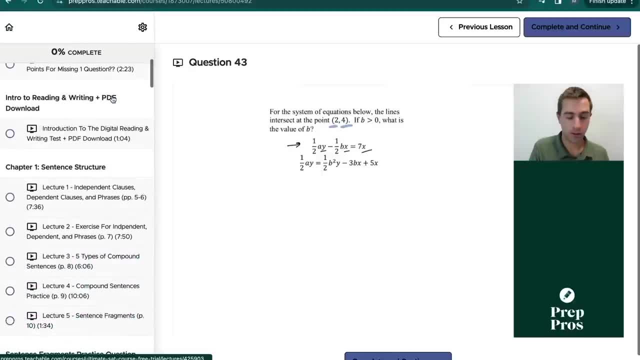 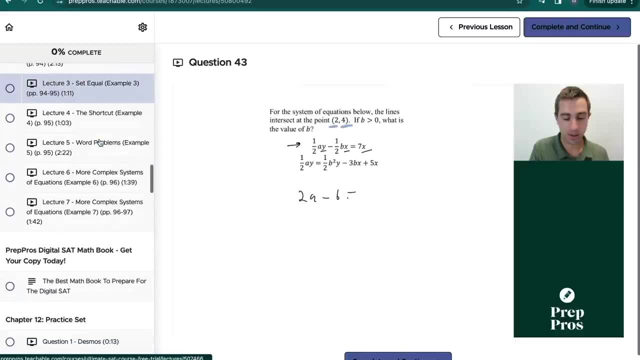 It's backed by a 100 point score improvement guarantee, So I would strongly recommend to check out the free trial. You don't need a credit card. You're going to get a few free hours of content. You're going to also get access. 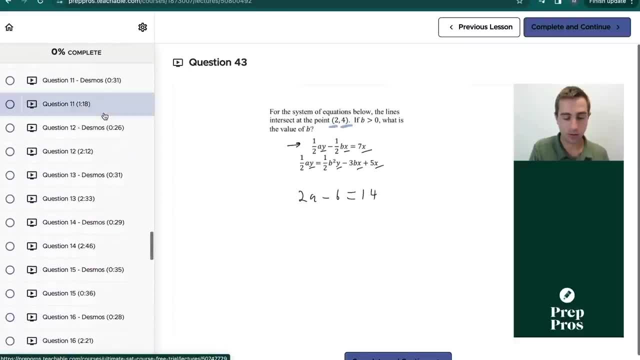 to the entire systems of equations chapter from our new updated SAT math book and all of the lessons and Desmos tricks that I teach there, which is one of the most important ones to learn. You're also going to learn some really important grammar rules. 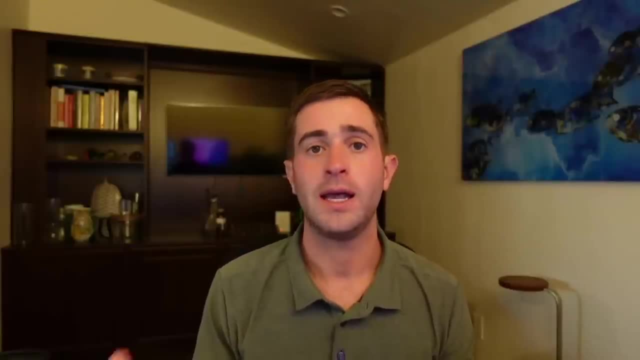 So if you want to check that out, you can see the link below, And I really hope this helped you out.